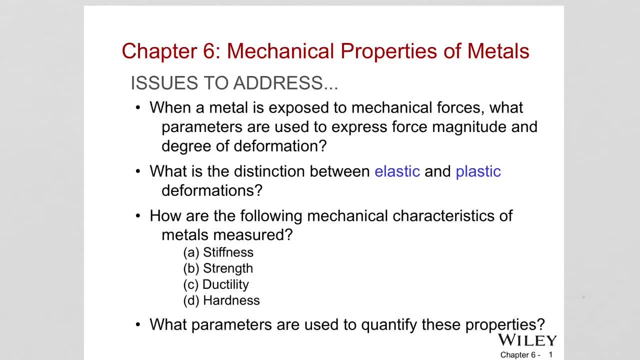 applied, how much it will deform or when it will fracture, when it will fail. so those questions we gonna answer- and some of you might have familiar with these topics because I'm sure you have seen these in other classes maybe- and we're going to see the difference between elastic and plastic deformation. what is elastic? 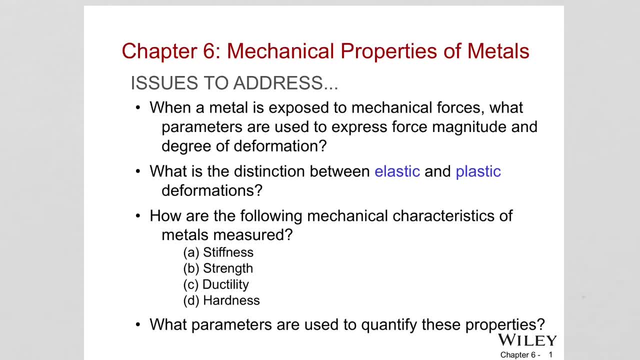 deformation. what is plastic deformation? so how are the mechanical properties are measured? so we're gonna see different types of tests that are used experimentally to determine the mechanical properties of materials, and I suggest you guys also watch the videos that i provide, because all those videos will show you. 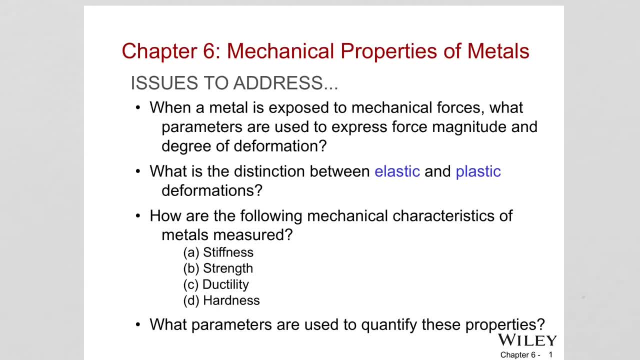 how those tests are done. if you are interested, you can also watch those. so when we say mechanical properties, these are stiffness, strength, ductility and hardness, and how are all those measured? okay, so different types of tests are being used to measure these properties. so which parameters are actually used to quantify these? so when we say ductility, which parameter we are going to? 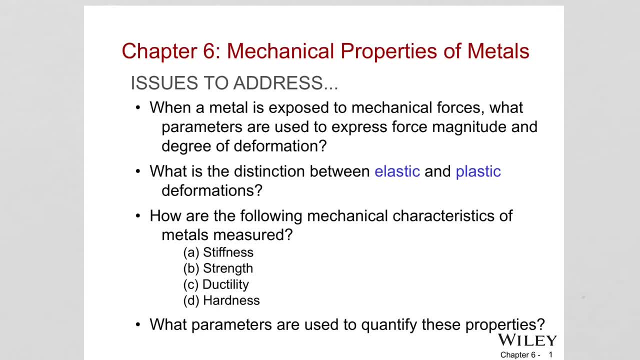 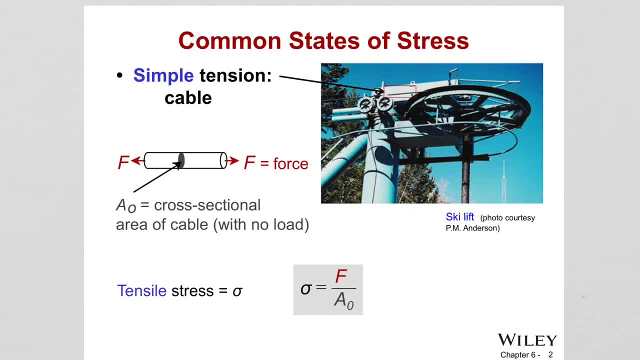 using we are using to say the material is ductile or not. so what are common states of stress? what type of stress is basically the materials are exposed to? and the most common one we call tension or tensile stress and we show it with sigma. you can see a part here. 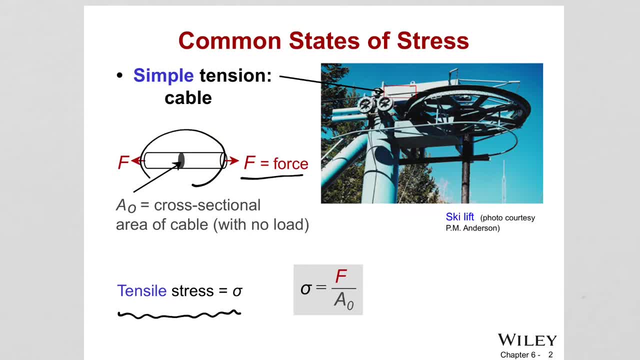 which is exposed to forces, uniaxial forces, meaning along one direction, like we are pulling the material from both direction. so the material, we say, is exposed to tensile stresses. so the cross-sectional area of that bar is a knot, okay, or the cable is a knot, of course the cross-sectional 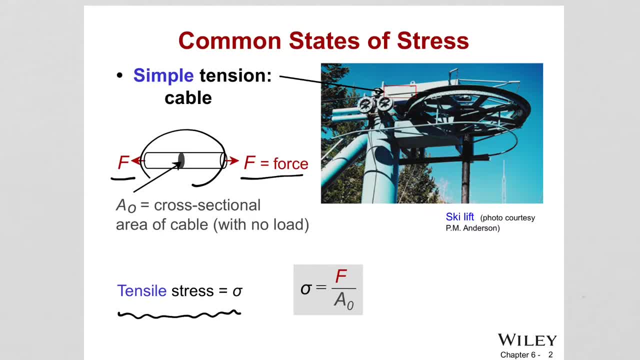 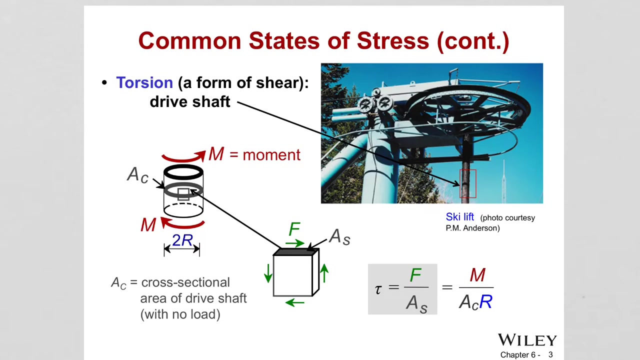 area will change as we keep applying the load, like it's gonna get smaller and smaller. but initial is a knot. okay, this initial starting cross-sectional area is a knot. so how do we define the stress? this is like pressure, right? so stress is force over original cross-sectional area. another type of stress is torsion or shape. 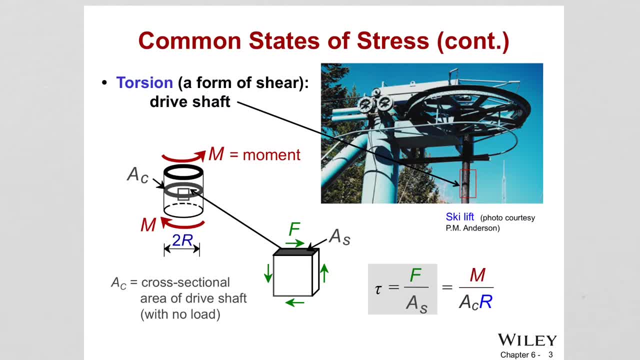 here, okay, where there is a drive shaft, for example, the part the material is exposed to torsion, like twisting as you go. see, here we are trying to twist the material on both sides and there is the torsion moment. here we are seeing torques and the cross-sectional area is 2r, the cross-sectional 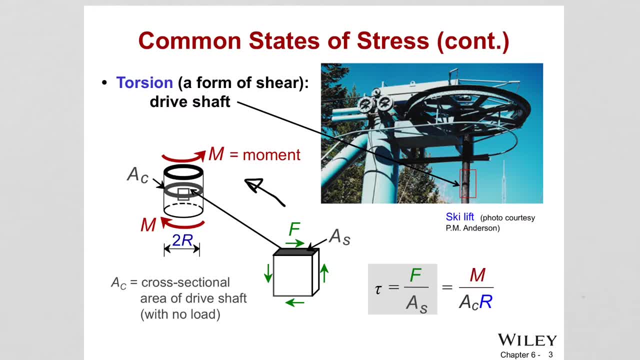 diameter is 2r, the cross-sectional area is AC. okay, and AC is the original cross-sectional area. so the shear stress here is defined as, again, the force over area area, if you look at the small unit within this shaft, or the force over area, if you look at the small unit within this shaft, or 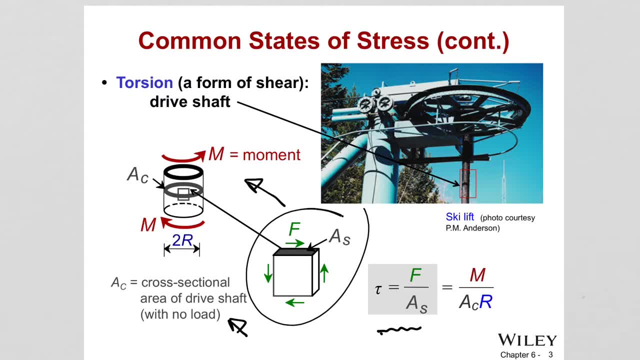 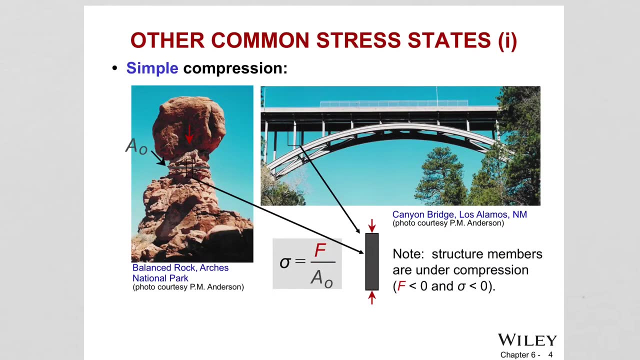 you can write it as: instead of force, you can say moment over the radius and with the original cross-sectional area There is also compression stresses, right, when we are trying to compress a material- This is the formula- is the same as the tension. basically force over. 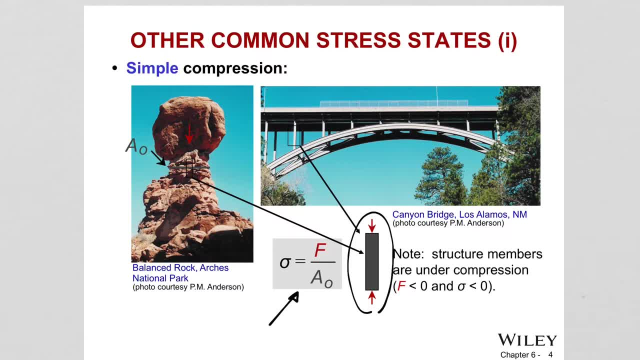 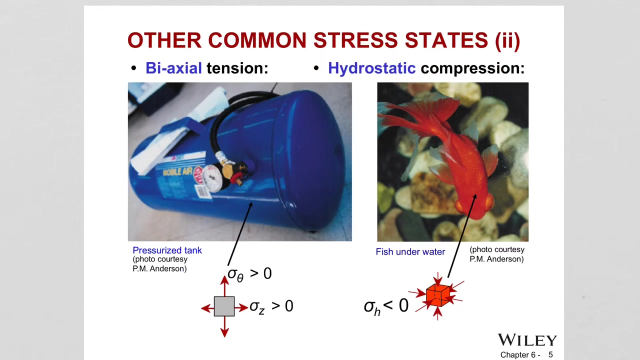 area defines the stress and many different parts are exposed to compression, like parts that we use in bridges, rocks, etc. Pressure tanks are exposed to basically biaxial tension. Basically, tension happens in two directions: transverse directions and when we look at the pressure, it is. 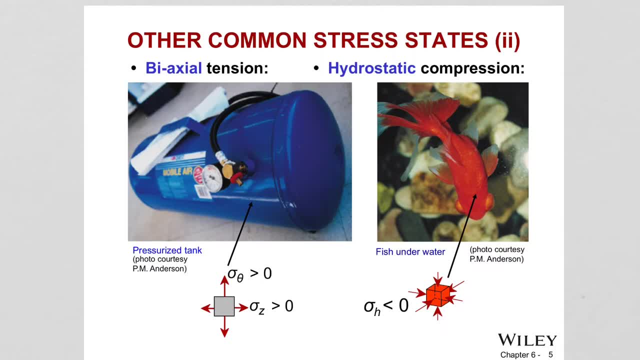 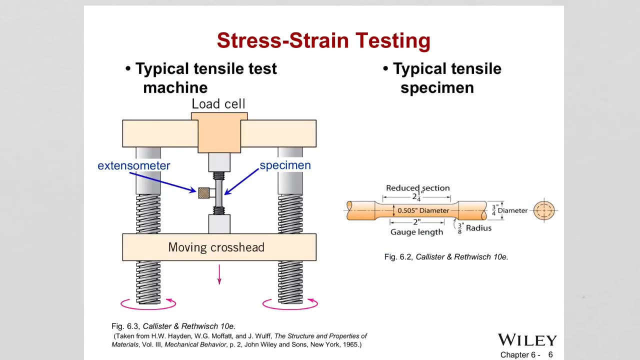 pressed in every direction Right, so we call that hydrostatic compression In 3D. in all directions there is stresses on the animal. So those were examples of different types of stresses the materials are exposed to, and the most important one is the tension. 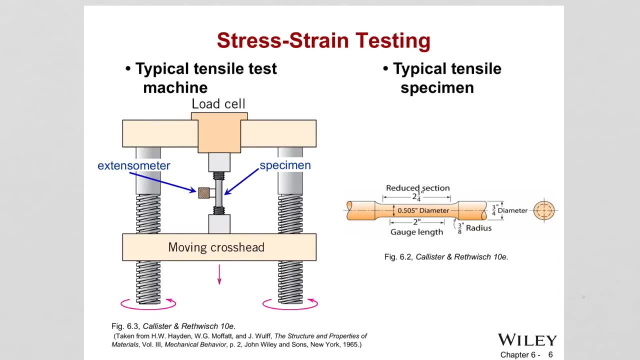 So the most important one is the tension. So the most important one is the tension. And how do we measure how the material is reacting towards the tensile stresses? We have tension tests we perform to be able to determine the properties and to perform this testing- we call it also stress strain testing- We need a specific 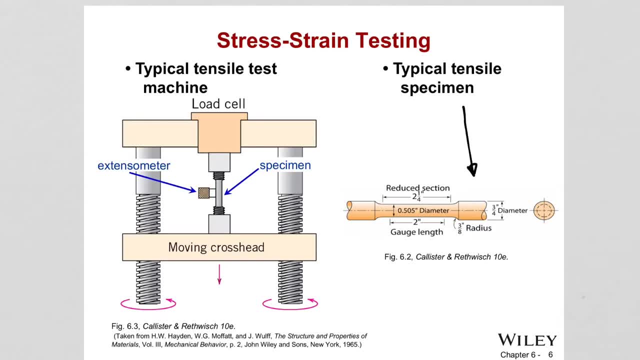 specimen, and specimen needs to be prepared in this shape, where there is reduced cross section and we measure a gauge length, where the gauge length is where the deformation will be observed and that specimen is fitted in the device, The device will pull basically the part uniaxially in both directions. 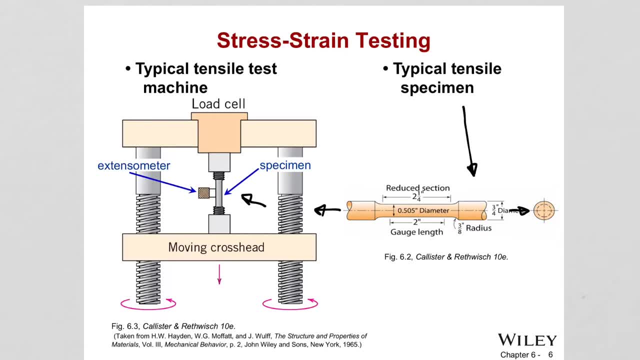 Okay, so specimen is placed. there is extensometer, which is a sensor detecting the deformation, Because when we actually pull the material in both directions, the material will start to get longer right, Extend or deform, or we call it strain, It's gonna change dimensions and then extensometer is able to measure. 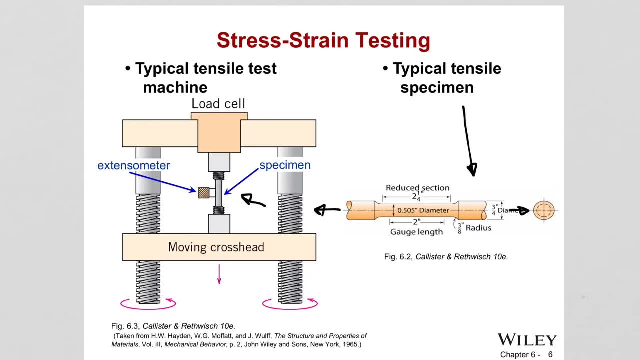 extensometer is able to measure, and then extensometer is able to measure, and then extensometer is able to measure, and then we measure that change. so in this test what happens is the machine applies a constant, constant deformation rate, meaning every second. let's say, I'm gonna make it up. 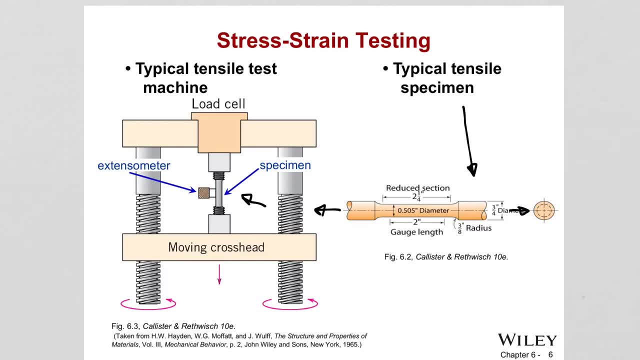 okay, every second it is trying to deform the material. let's say, 10 millimeter I'm making okay. so, basically, the deformation rate the device is trying to keep that constant. okay, and then what it does is it records the force that it needs to apply to keep that deformation rate constant. so in with time, of course, the 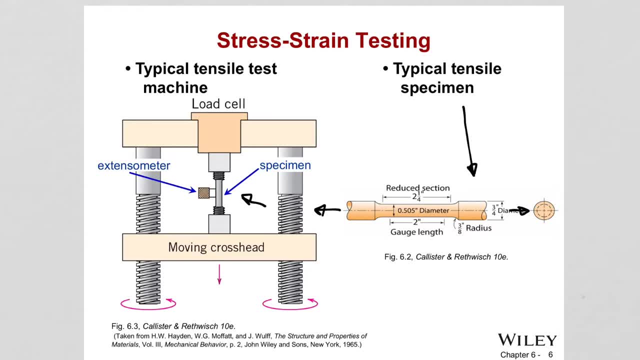 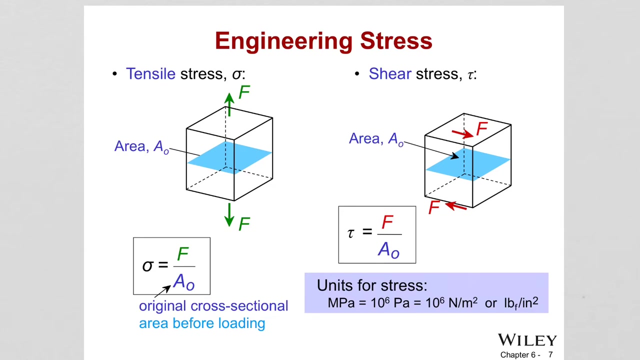 force will change. as the material keep deforming, less forces might be necessary to deform because it will deform more easily. so what I'm trying to say? it will keep the deformation rate constant, but measure the forces, measure the deformation and then calculate the stress and strain. from the equations we're gonna learn. so 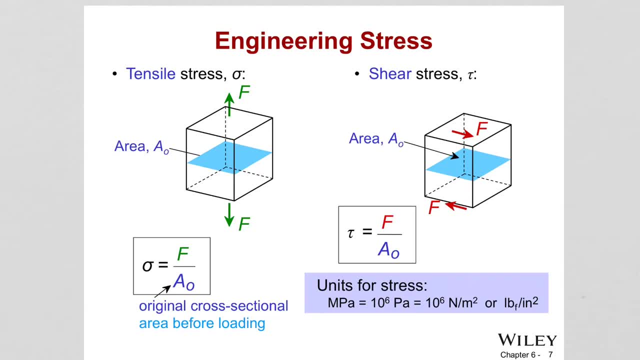 what type of stresses, the material, or it's possible we said that tensile stress, which was the signal, which was force over original cross-sectional area, and the shear stresses are acting along the surface like that, trying to share, and the shear stress is also force over the cross-sectional area. it is acting when, when we defined the stresses, который hiện. 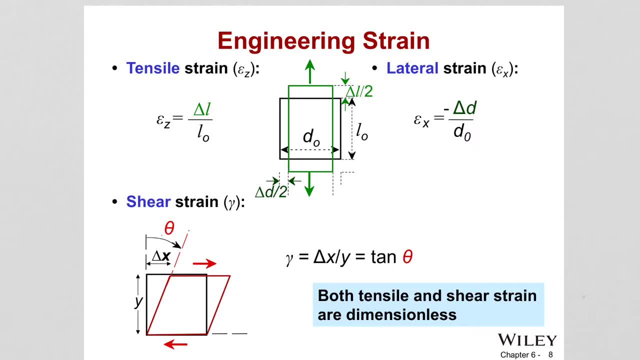 nach an услов活为. When we define strain engineering strain is shown with an epsilon subscript z, meaning the deformation is happening along the z direction. But actually, when the deformation happens at z direction, let's say this one we have here right. 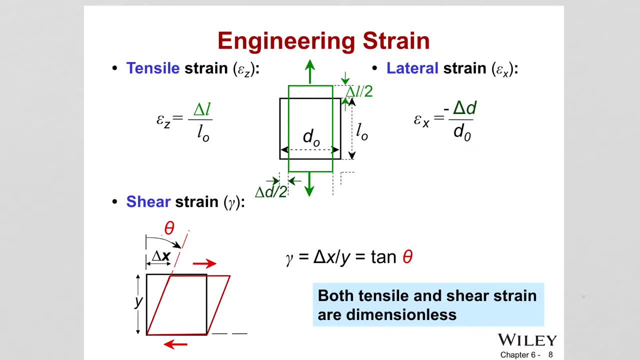 And no, not this one. So originally let's say we have this one right And then we pull this And when we pull the mid part it's going to elongate. But when it's elongating in z direction, in the lateral direction, it will be exposed to acting like it is compressed. 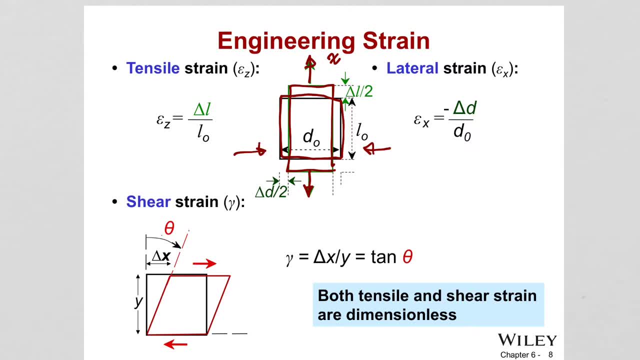 It will get smaller. Okay, so therefore, if you're going to define the deformation, you need to be careful in which direction you are defining that. So in this case, strain Or the deformation with tension along the z direction, is shown with epsilon subscript z. 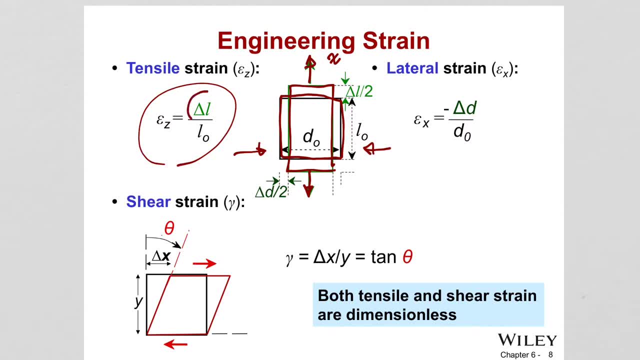 Which is equal to the change in the length, which means the final length minus the original length over the original length. Okay, so this is showing us the strain And if you're going to define the lateral strain, which is the deformation in the transverse direction, 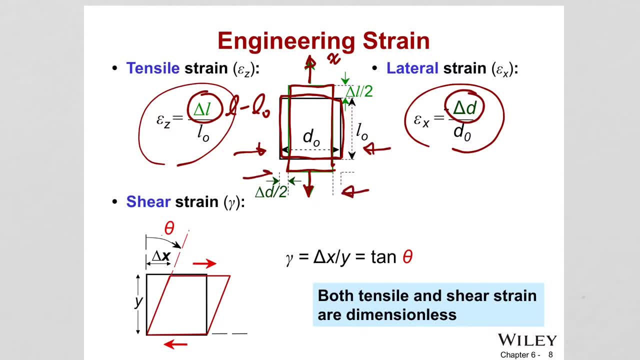 so this is the deformation in t. So this dimension is like maybe diameter right, So shown with the d. So delta d over d naught, So delta d is final diameter, let's say minus original one over the original one. 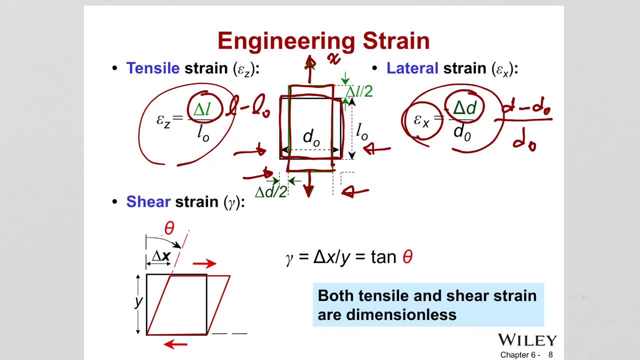 So this is the deformation strain along the x axis, But when we usually define engineering strain, it is the one that is along the z direction. of course, shear stresses will also cause deformation in the material, just like here. if we expose the material to shear stresses, the material will deform, like this. right, so it will. 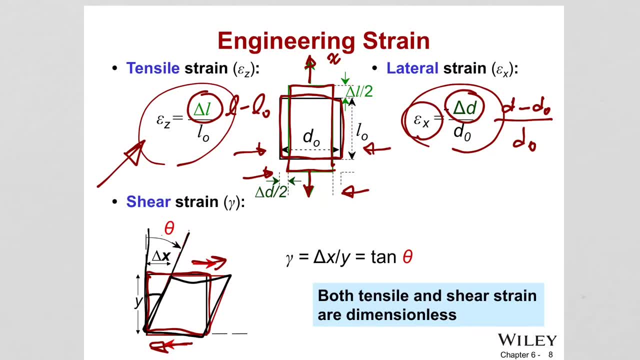 make an angle compared to the original starting point here: theta, so the tangent theta is actually how we define with the gamma, the shear strain, shear deformation, that is, Delta X over Y. all strains are dimensionless because at the end we are dividing length to length or diameter to 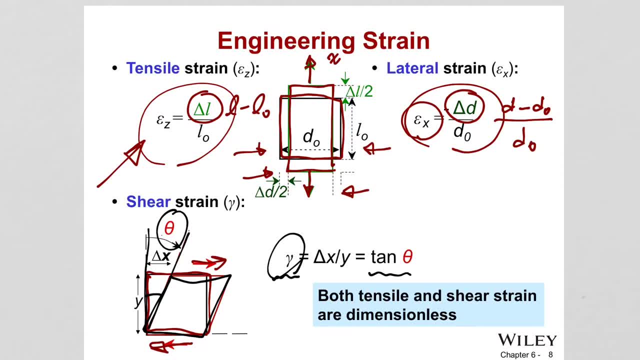 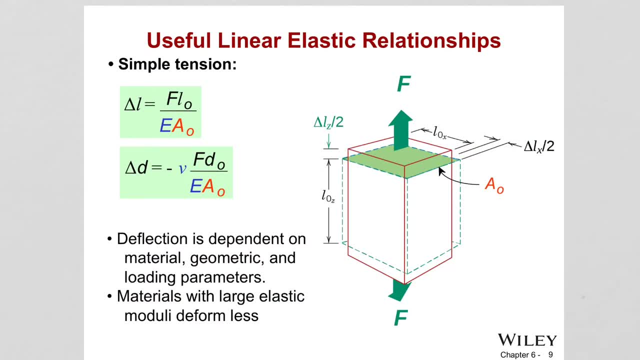 diameter, so the units cancel. so when we say strain, strain is something dimensionless. so materials deform elastically and plastic, this whole elastic deformation, is the deformation. so when we release the forces the material can go back to its original shape. so it is reversible and you can recover it. so when the material is deforming elastically, there is a relationship between the material and the shear strain. so so this is because the force 0.2 degrees deforms. so if we do the force positive or negative, force 1, then it is something deformation that will make a base. Deep Valleys projecti will be formed. 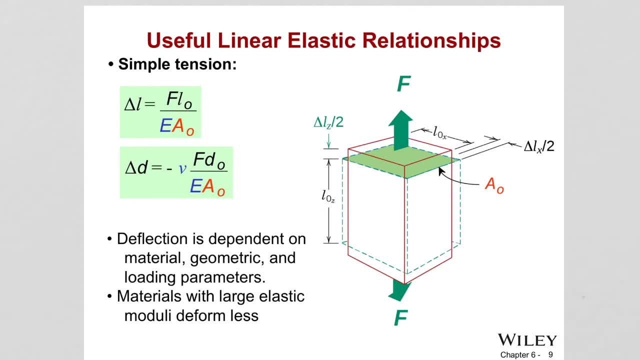 So we corrections that defarannce, that changes support ceil. вот, I will see later. Relationship between the stress and strain. Strain and stress are proportional and the proportionality constant is defined by elastic modulus or Young's modulus. We showed with a symbol E. 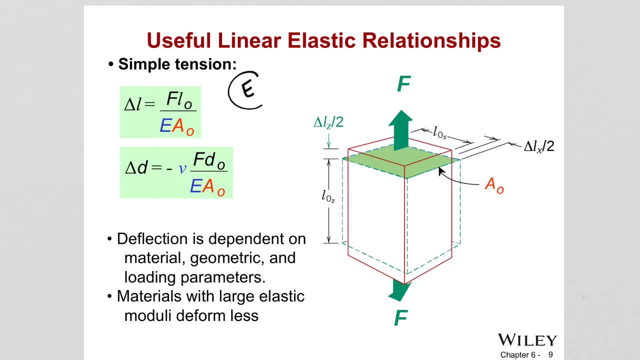 So this Young's modulus or elastic modulus is the property of a material. Basically it comes from the atomic bond strength. So if material resists to elastic deformation it means it has large elastic modulus or Young's modulus, It means the atomic bonding is strong. 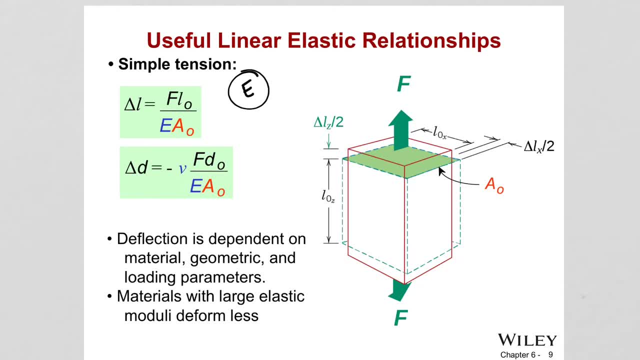 And we see it is so strong that it is not elastic. We saw that parameter when we were looking at atomic bonding We briefly mentioned, And so this linear relationship between the stress and strain is defined with. the modulus is equal to stress over strain. 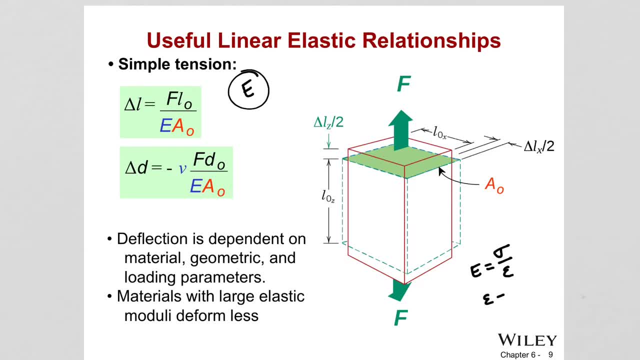 Or strain is equal Or strain is equal to stress over modulus. So because when they collect the data from the tension test and they remember, they measure the force and the device and from the force they divide it into cross sectional area and the test equipment, giving us this curve. 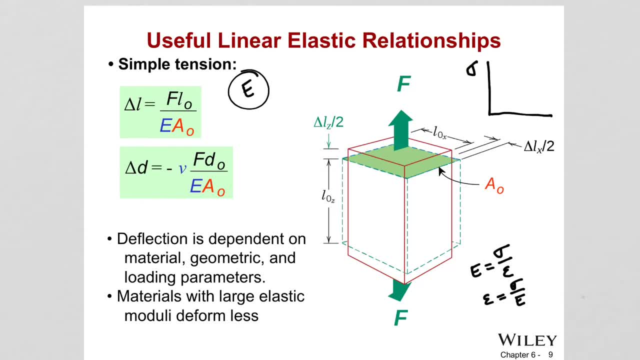 We call this stress strain curve. And then on the y-axis we have stress, On the x-axis we have strain, And when initially always the material deforms elastically, that means a recoverable deformation. there is a linear relationship. The material behaves like that. 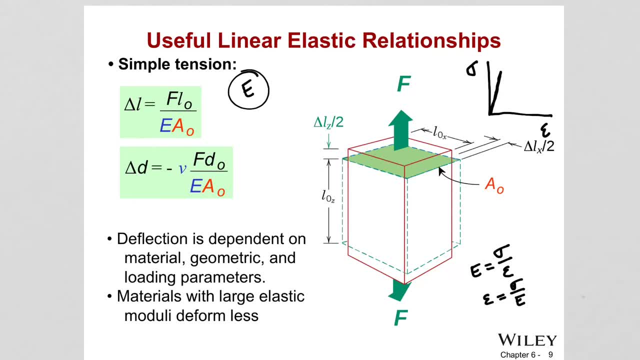 So stress and strain proportional and the proportionality constant is E, Or this is also the slope of the strain stress curve. Okay, So when we understand Young's modulus and the origins of it, I told you guys atomic bonding. If we say material is stiff, that means the material has a high modulus. 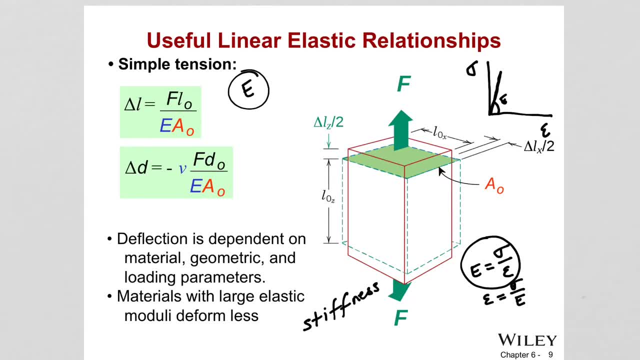 Okay, Stiffness, And if it's like a rubber, for example, easily deform- Easily deform, to a large extent elastically- then the Young's modulus is low. So, for example, For metals, ceramics, the Young's modulus is high. 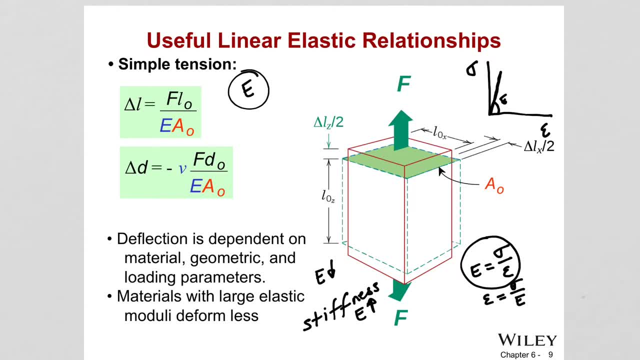 For polymers like rubber, the modulus is low, It can easily deform. Okay, So how do we obtain some correlation between these equations? So we said strain is stress over modulus E, Young's modulus, And then This is also equal to. we learned: strain is delta L over L naught. 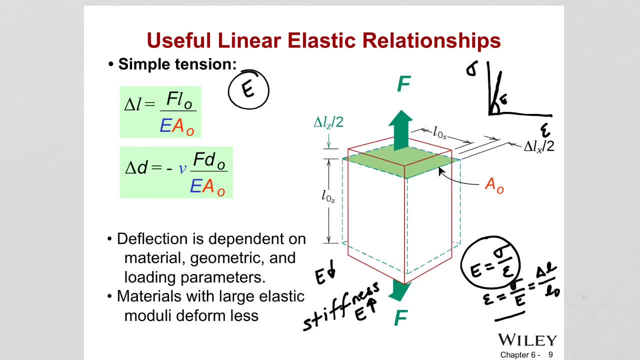 Okay, So I come to here. So I know this. I know the stress is stress. Instead of this stress I can write force over cross sectional area And there is E which is equal to delta L over L naught. So this gives us delta L as force times L naught over area times. Young's modulus. 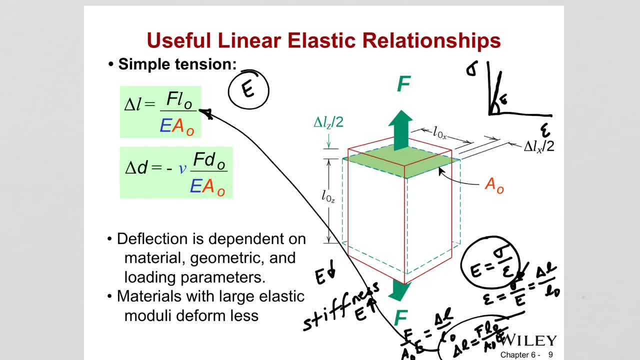 Okay, So this is that equation here Which tells you, besides the force and the Young's modulus, Beside the force and Young's modulus, The geometric parameters, And Will determine the deformation, Because delta L is telling how much length change. 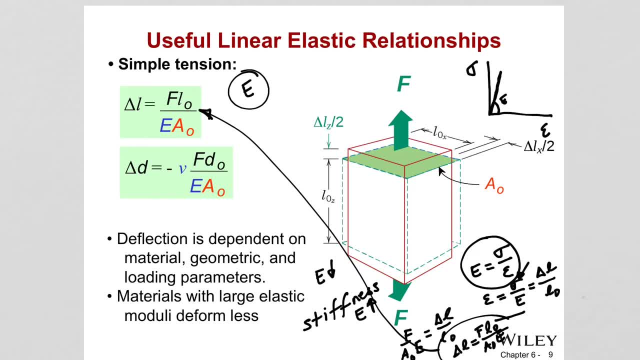 Like the deformation, Right? So We see that from this equation, Okay, Okay. So let's erase everything on the screen And look at the second equation here. So There is a property called Poisson's ratio. We show it with the symbol V. 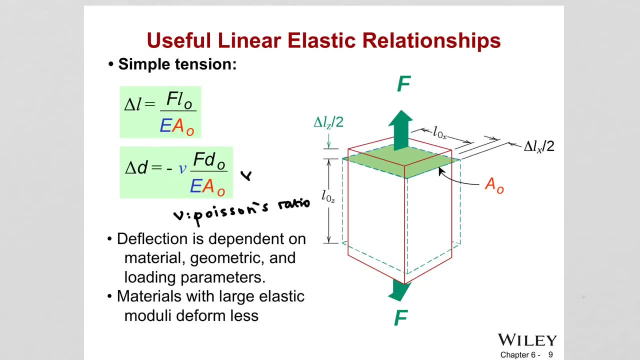 This is, by definition, Poisson's ratio. V in this equation we are seeing Is equal to The lateral strain over The Z direction strain. Okay, And there is a minus sign. The reason is When we elongate the sample in the Z direction. 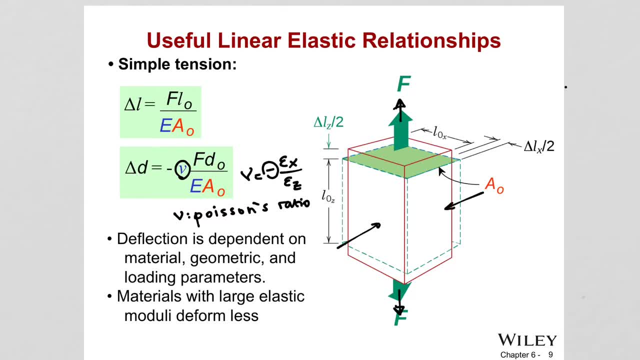 Remember it is compressed in the X direction, In the lateral direction, So it is actually There is a negative change. The strain is actually negative Because it is not elongating, It is under compression Right, It is contracting, So this is negative. 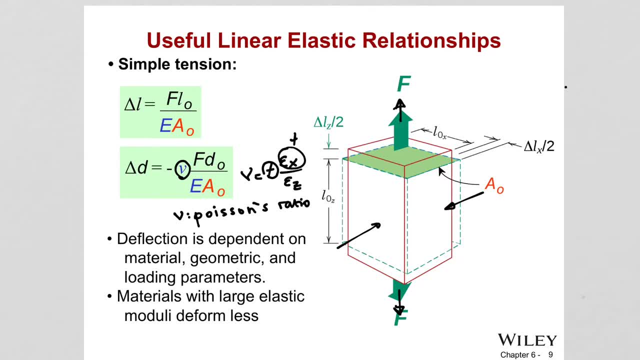 This: With this negative, It is the making Poisson's ratio positive. Okay, So by definition We said Poisson's ratio is AX, The epsilon X over epsilon Y, Or Epsilon Y over- I'm sorry- Epsilon Z. 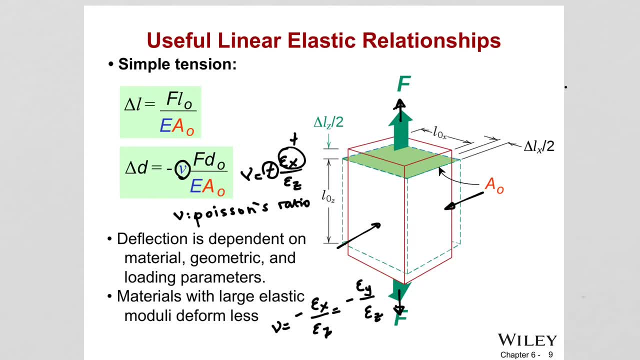 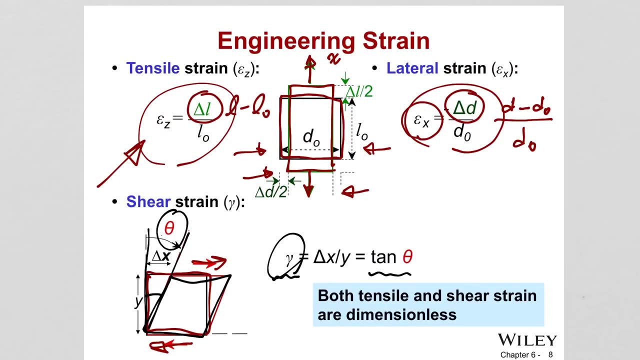 Okay, So The lateral deformation, The Delta, Delta D, We Defined it Along the X Axis. We said: Remember, Epsilon X Is equal to Minus Delta D Over. 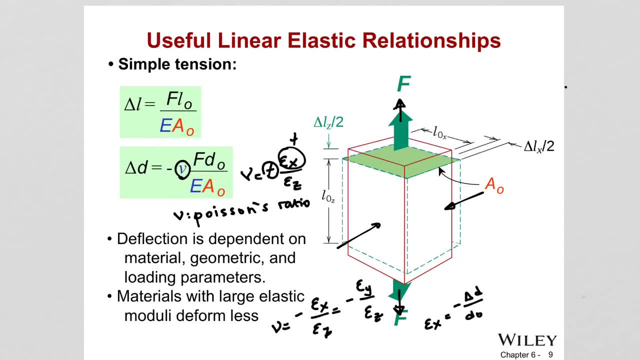 D naught. So This is Poisson's ratio, How it was defined, And instead of Epsilon X I can write Delta D Over D naught. So The negative sign Here Is again. 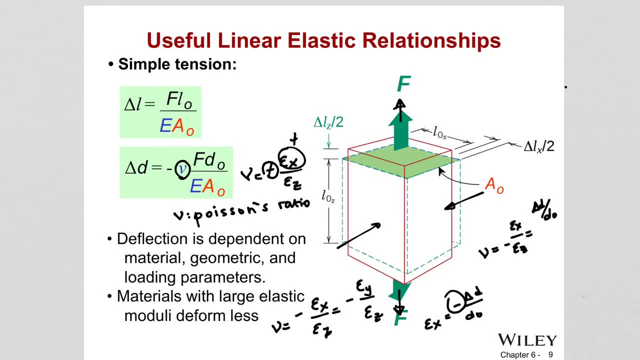 To make strain positive Because It's negative. And we already Accounted For that By putting minus In the Poisson's Ratio, And this one is Delta, L Over L, Not Okay. 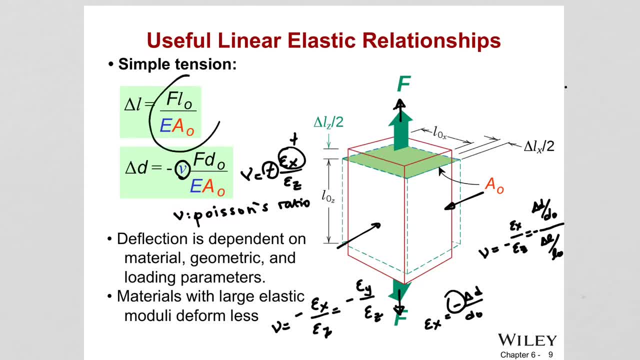 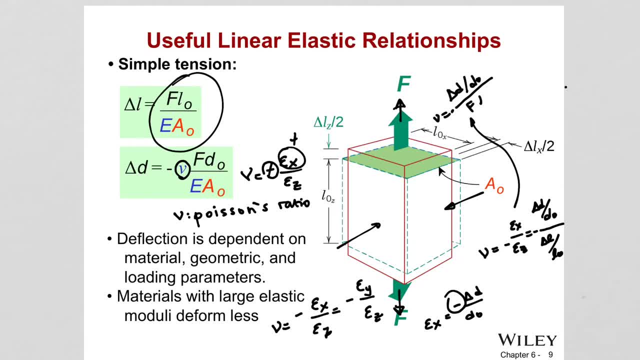 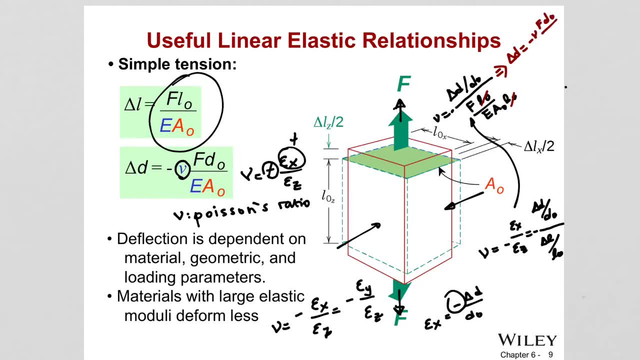 F Times D Not Over. F Times D Not Over E Times A Not Right. So That Is This Equation Here. So Basically It The Dimensions. 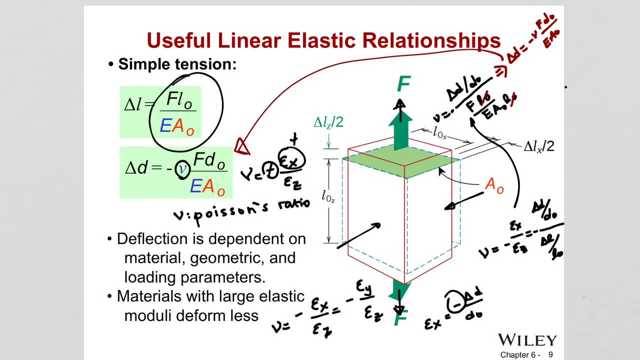 Of The Basically The Material. Okay, So We Learned Here What Is Poison Ratio And And Do You Guys Know A Material With A Poison Ratio? 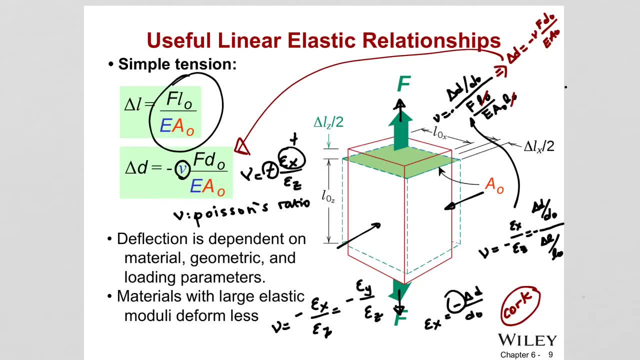 Of Not A In The High, The Out, In The Col Portion, In The In The Out, To Be The Dimension. It Does Be Hard. 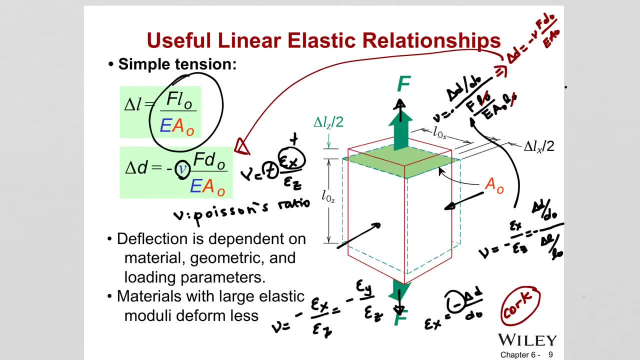 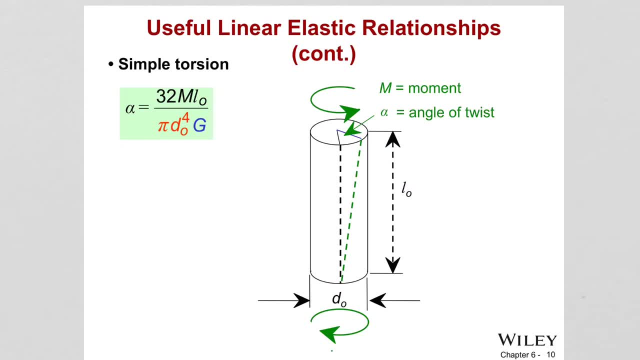 Push In The Spot, So That slide. there is also another useful relationship to explain torsion, which is angle of twist. that is related to this torsion strain. so this bar is exposed to torsion. right here we are trying to twist it and if there is, let's say we 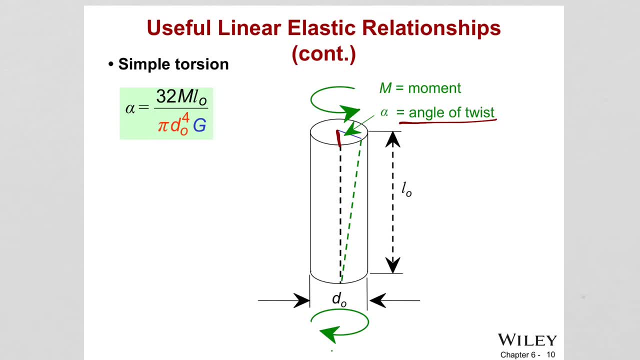 put a sign here like that, okay, and we cross the sample like that, and then we, if we try to twist, that line will come here. so there is the angle in between, called angle of twist, and that shows us how much the material is deformed. and this relationship is given to us here, but I'm not gonna ask anything about. 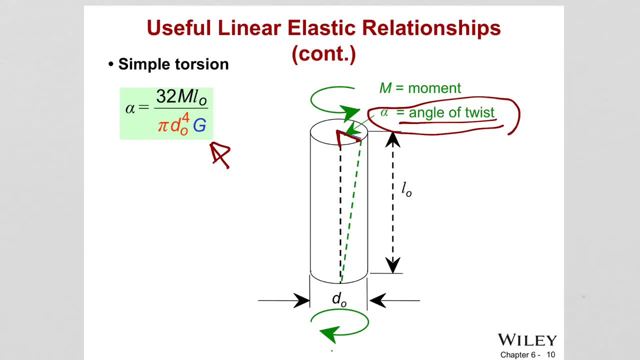 torsion. you just give the line, the angle between the two places for seeing the torsion. just give the line, the angle between the two places for seeing the torsion. give the line, the angle between the two places for seeing the torsion. you this information so that you guys can keep it in mind in case in the 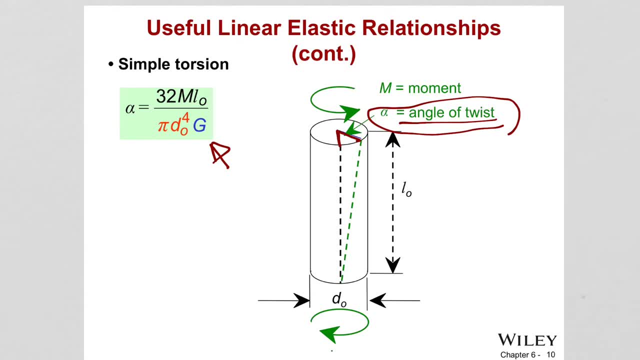 future you can, you might want to use it and come back. you can see this equation here, which the angle of twist is basically related to the deformation, and that deformation is again related to the moment dimensions and G. so here all we understand from this chart, the important point we got to understand. 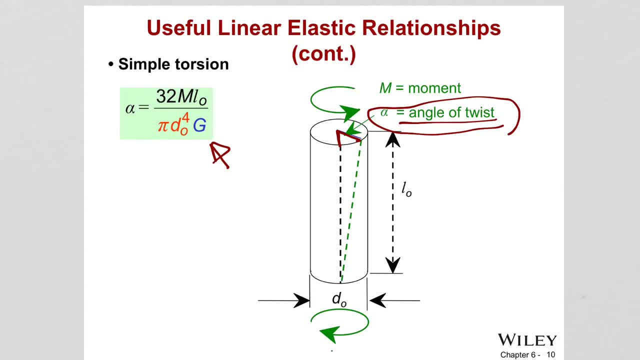 again, the deformation is related to the forces apply and then the characteristics of the material, and then the dimensions and the characteristics of the material previously shown with Young's modulus, when we were working with tension, but in torsion, when there's twisting, we talk about G. G is basically shear modulus, okay, so let me write it down. so: shear modulus. 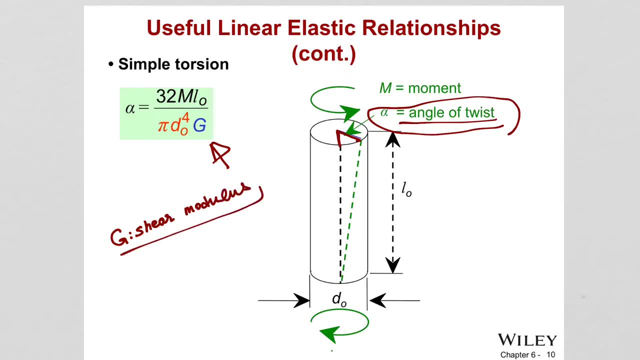 which shear modulus can come in the exam. okay, this part is important. so how we relate shear strain to shear stress is: with the shear force it's decomposed stress that 실ICES the area much. so here we're going modulus. so normally when we have tension it was stress. normal stress was equal to. 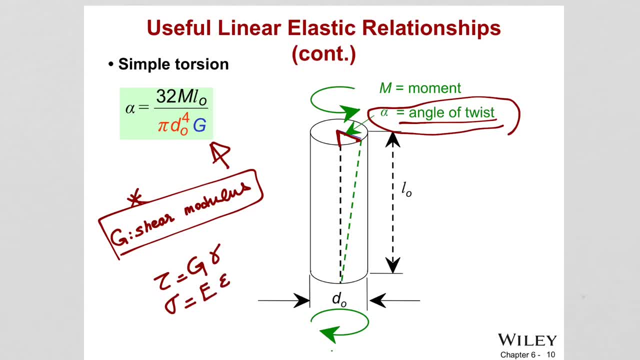 modulus and normal strain. so in that case, this is. these are the same things, but instead of Young's modulus here we have shear modulus, because this modulus is related to the shear, so that's why we use it with a G. we symbolize it with G, okay, so G is important and, of course, this is. 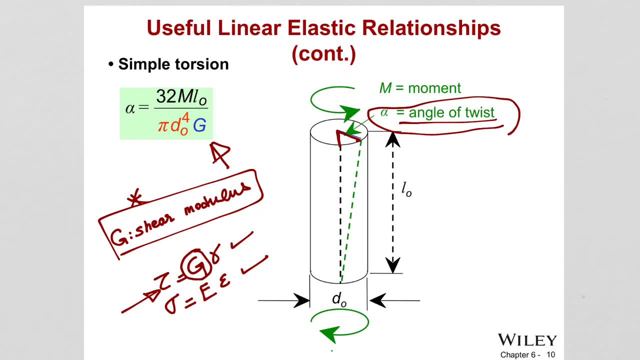 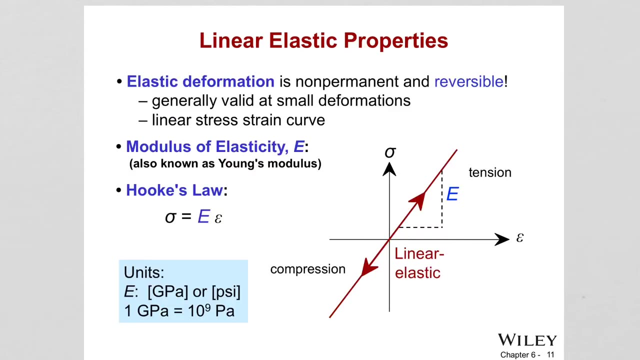 again a linear relationship explaining elastic deformation under torsion and the explaining relationship between the shear strain and shear stress. alright, so we said elastic deformation is not present and reversible. think about: you have a rubber band and you stretch it and when you release it it goes back to its original shape, right? so this is what we call elastic deformation. 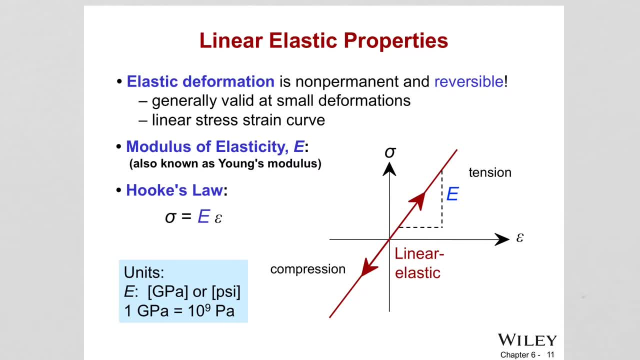 and this happens at small deformations. okay, so at large deformations, when you release the forces, you might not be able to go back to the original shape, such as your, let's say, you have an aluminum foil, you bend it and when you release the forces it doesn't go back to its original shape, right? 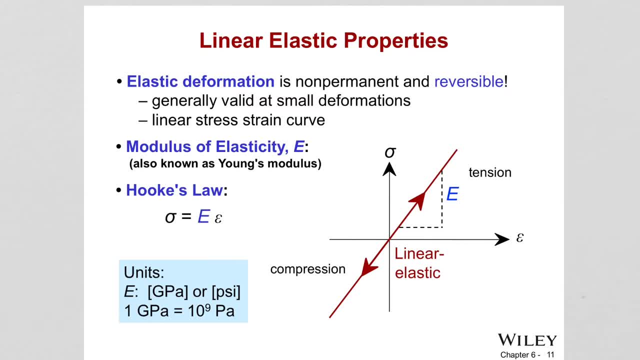 so, when we are talking about small deformations, usually this is called elastic deformation and it is not permanent and the relationship between stress and strain is linear, as you can see. here is a graph of strain stress versus strain, and i showed you, guys, that under tension, this is. 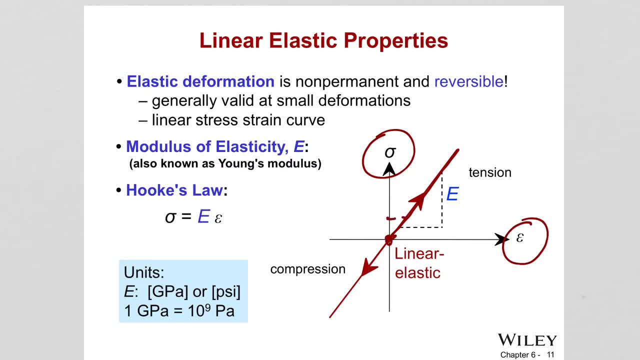 linear increase, how stress is increasing with increasing deformation. okay, so device was measuring force and was dividing into area and calculating the strain and also measuring the deformation and calculating the strain. this was stress, this is strain. okay, it's confused. okay, so the slope was gonna give you the modulus right, e and 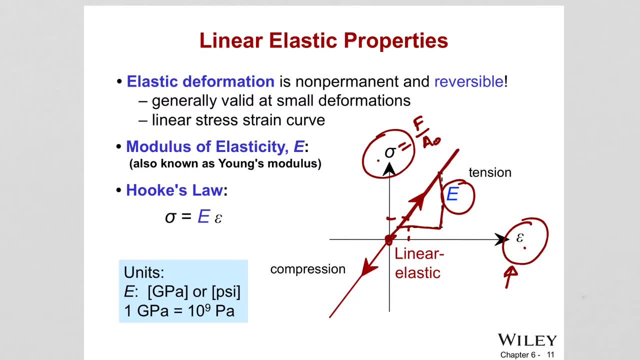 okay, and when there is a linear relationship, e is constant. you can see, guys, okay, e is constant throughout this deformation, and this is called young's modulus, or modulus of elasticity, and the linear relationship is called hook's law. that relates the stress to strain, and i showed you this one, guys. so 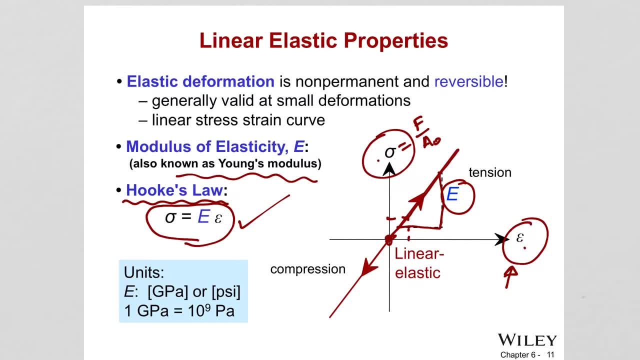 what is the unit of modulus? because this one is unitless. the unit of stress and unit of strain is when it is았a factor of the modulus is equal to eg, it gives be ferร quiereito. it's a formula of mass right. so in región of the modulus is the same, which is ج or pascal, basically like pressure right. 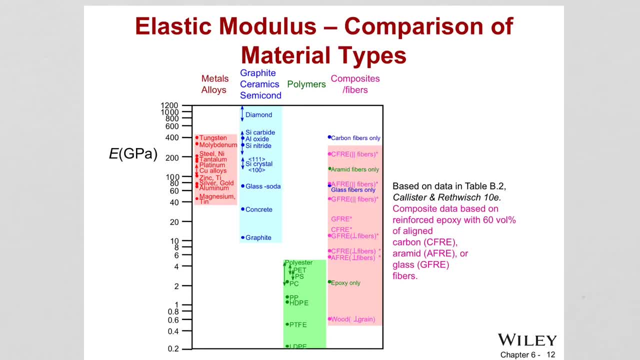 the yank SS b Delius modulus and the yank danced it GIPAS, there's like 3. so you guys, to understand, as i told you, the young's modulus is characteristics thereуб to be like لم. may you all be OK. property of the material. and it's the change, the panning, and what type of material you ha. 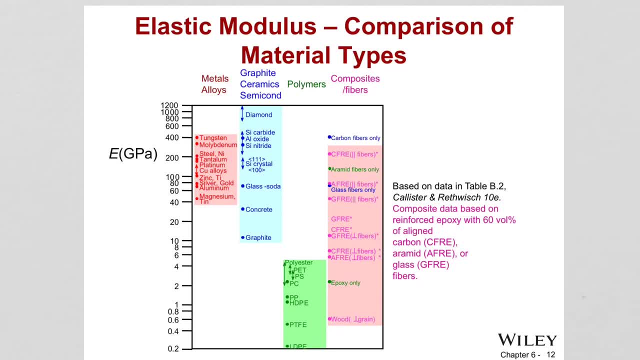 dining from the bondings on the democr celebrations. engineering region and illustrations has come from this following to anyway in political nonㄴ, atomic bonding between the atoms, the strength of it. therefore, we look at it, the highest modulus materials are ceramics, graphite semiconductors, because these materials shown with the blue here, 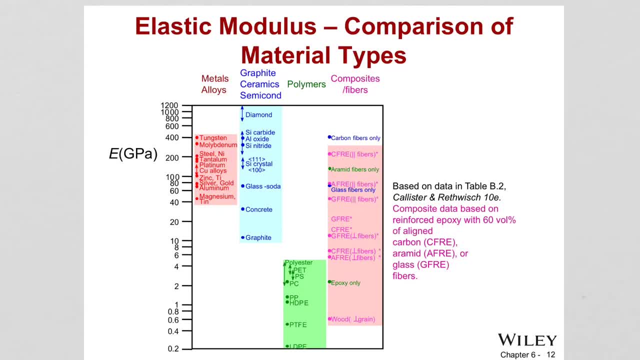 they have, like diamond, very strong materials, ceramics. they have ionic and covalent bonding and this, of course, it is very difficult to deform those materials elastically. right, think about you are trying to stretch diamond- how possible is that? and then, uh, that means they are very stiff. 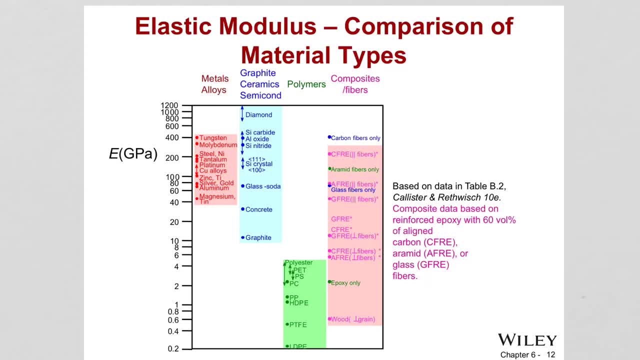 very stiff materials so the modulus for those are very high and besides that also the metals. metals are also the metallic bonding providing uh other relatively high, compared to polymers and some composites higher modulus values. so we can see tungsten has the highest because, i told you guys, tungsten has covalent bonding. 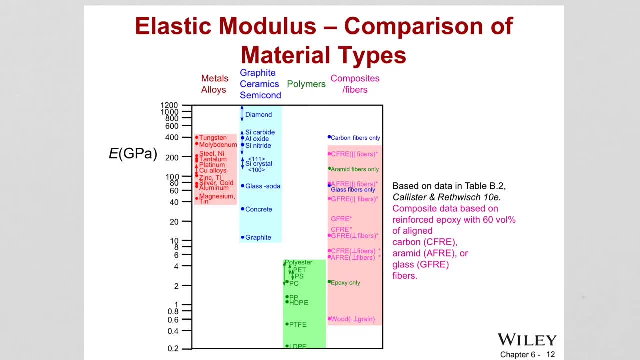 besides the ionic bonding and beside the metallic bonding. so it follows the molybdenum, follows that. steel, platinum, copper and ceosin. c10 and magnesium are the ones that i have the lowest modulus. that means they are easy to deform, like aluminum, right aluminum, easy to deform, you can easily deform an. 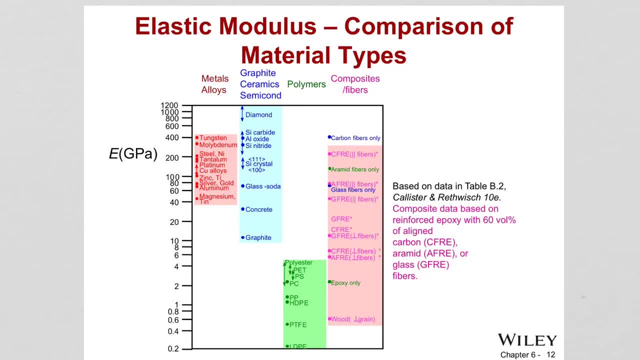 aluminum foil and aluminum bar. okay, so when it comes to polymers, polymers in between the chain, between the carbon chains, carbon carbon bond. carbon carbon bond is very strong, we know, but when we deform polymer. so remember, this is one chain, another chain of polymers in between them. 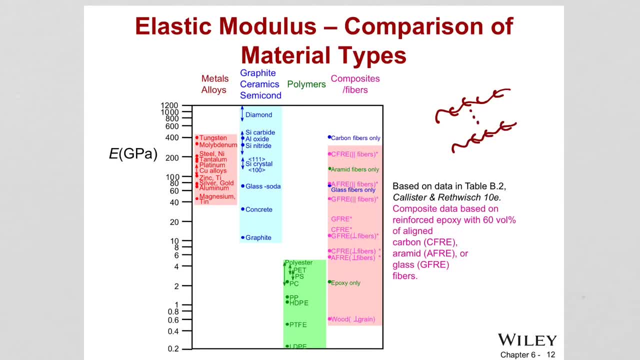 carbon bond, but in between the chains- not within the chain, but in between these chains- we have weak bonds. so when we try to deform the material, actually these weak bonds are broken, not the carbon carbon bonds. that's why you might expect polymers, because of these carbon carbon bonds, to have a 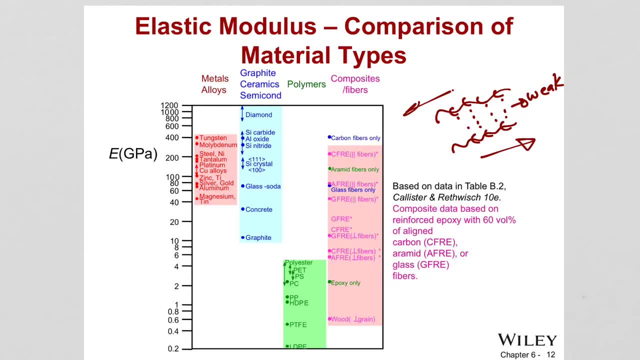 very high modulus but in reality they have the lowest modulus compared to other molecules, other materials. because of these weak bonds are determining the mechanical properties of polymers, so the chains can easily flow over each other. the material can easily deform. okay, so composites and mixture of two different materials. they are mostly made up of polymer. 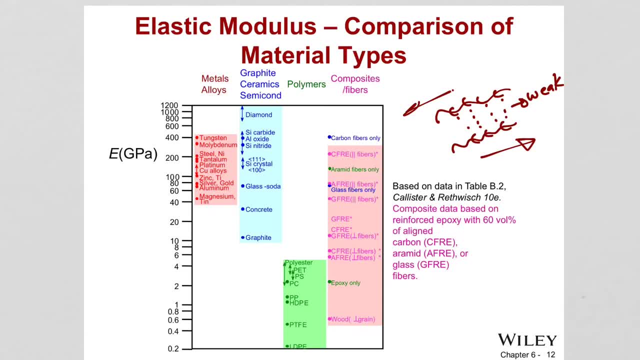 with the reinforcing fibers. therefore, it is closed. the modulus values are close to polymers and of course it covers a wide range, because composite means materials that are made by combining two or more materials so they can put fibers into polymer matrix etc. and this gives us a wide range of young's modulus values. 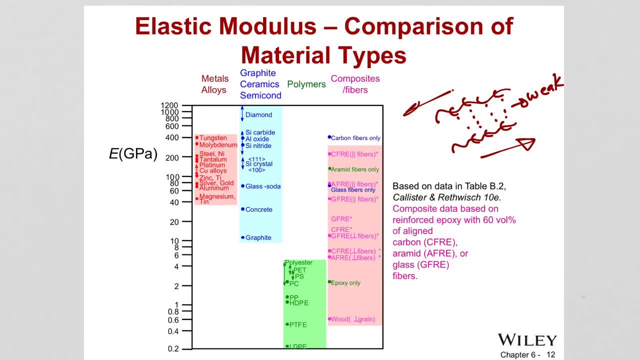 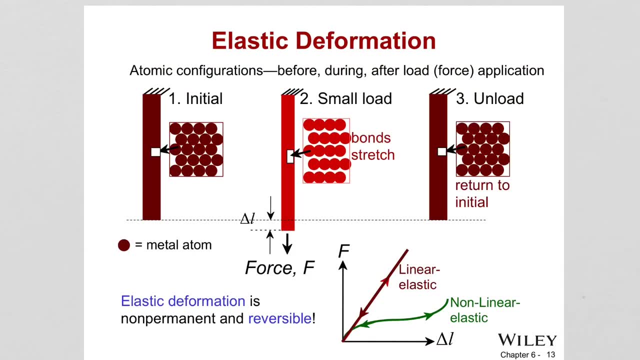 so this comparison between the moduluses of different materials, it's important to figure out which MAY be the most suitable to, Especially taking into account because these units were like three or four. so I have two samples I will show you in a minute, because this one only I have this one. 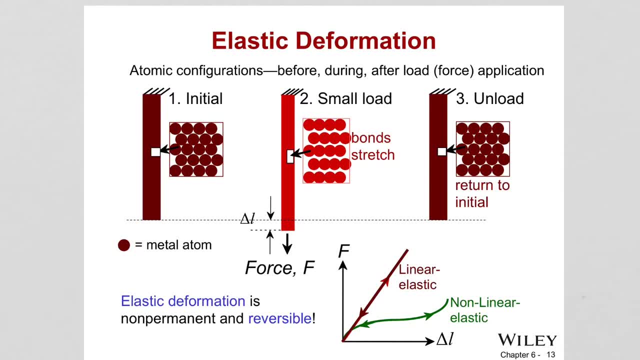 more model and for you, which I am doing, although you can see here, I have one more sample. this one is new, so this is the finally earth-based society model. so, yeah, the atoms are well packed and in number two, we apply the tensile force, trying to stretch the 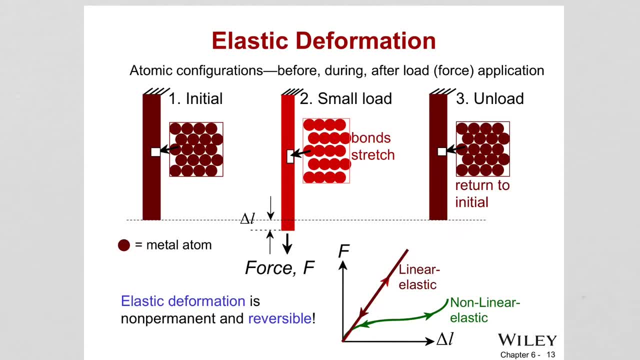 material. therefore, you are stretching the bonds, atoms start to separate always. i think about, think about, you know, the modulus or bonding between the atoms. think about them like there's a spring in between them and when you stretch this bond, it's like spring is extending right. so, in number three, when we release the load or unload, the atoms can move. 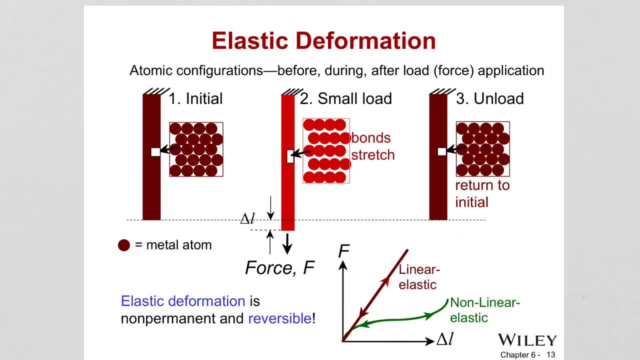 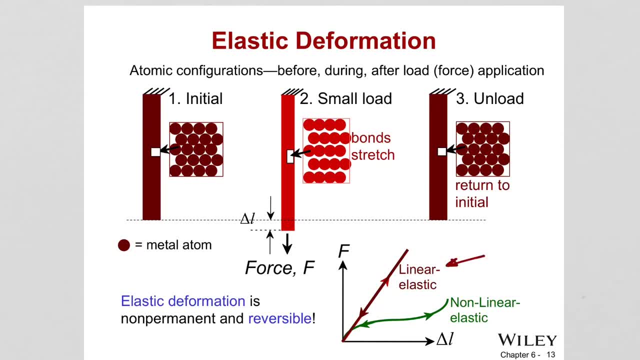 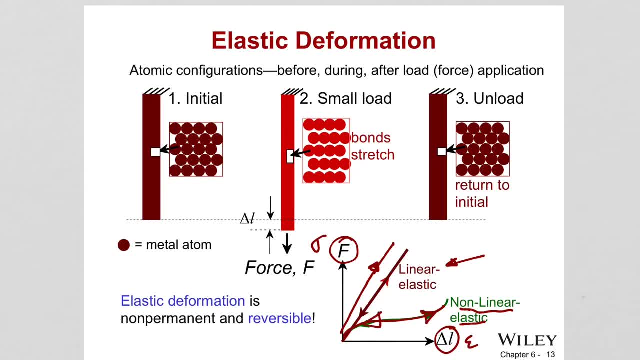 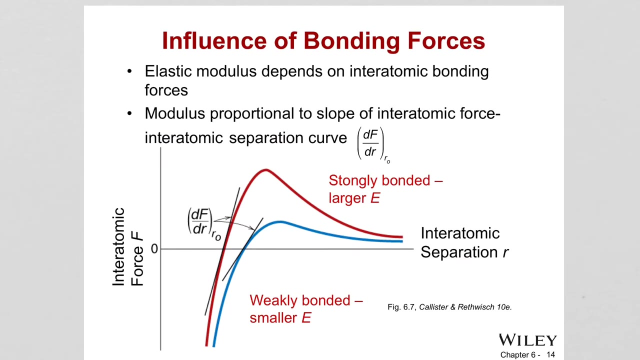 elastic and it can go back to its original shape. okay, this is like rubber behavior here. so so, mechanical properties of polymers, and it's a little bit complex compared to metals how metals behave. so, as i told you, the modulus depends on the interatomic bonding forces or strength, right? 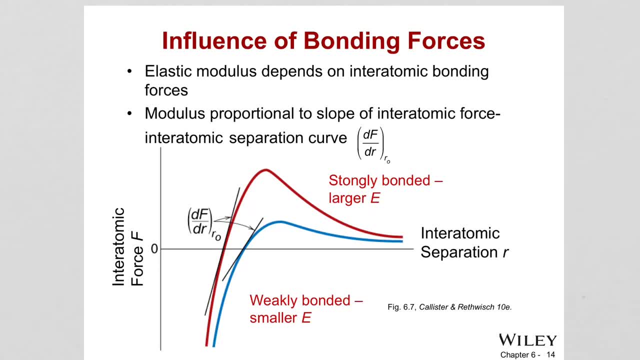 and it is proportional to the strength of the bonding forces and the strength of the bonding forces slope of interatomic force versus interatomic separation. so logically you can understand that right. how much uh you can separate the atoms with the applied forces? basically it's going to depend. 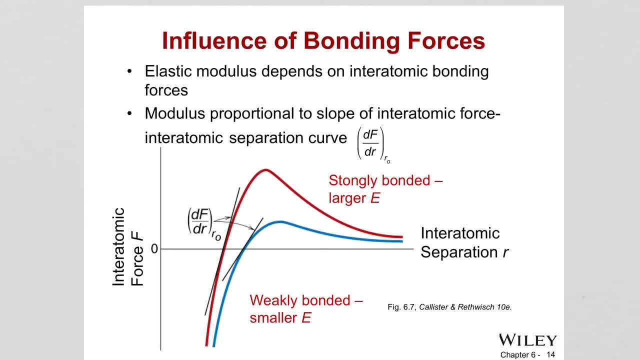 on the modulus. so basically, if you have this force versus separation curve, the slope uh at the um equilibrium separation distance is gonna give you uh is because you need it. at that point, right at a point the slope is gonna give you the modulus. okay, so the strongly bonded ones will have a bigger slope. 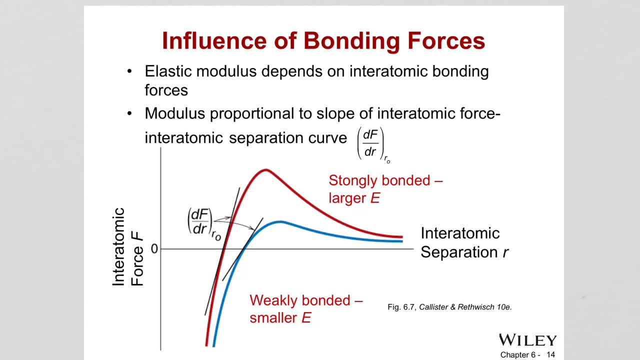 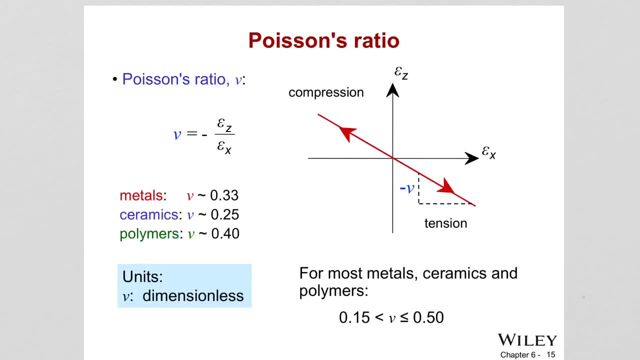 weakly bonded ones will have a smaller slope and smaller modulus. therefore, they will have a bigger slope and smaller modulus. so this is, as i explained, the poissons ratio, and it is again dimensionless. but here i think they made a mistake, because this should be right. but also it basically depends on, of course, 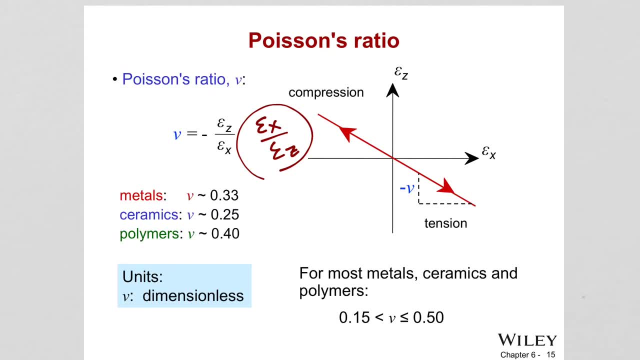 what kind of force is going to be applied between the yz, x-axis basically? but it should be the ratio of lateral deformation to the deformation along the tension. so we are given the general values for poissons ratios, and this is for most metals, ceramics and polymers. it's in between. 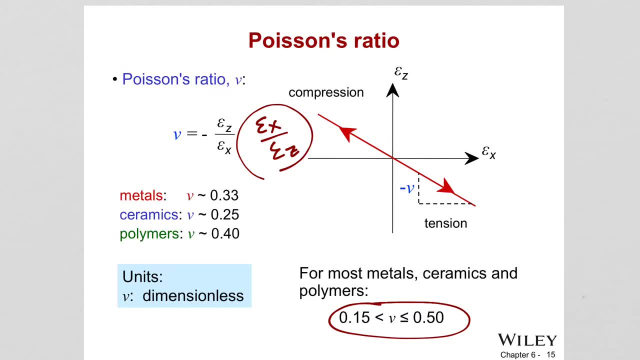 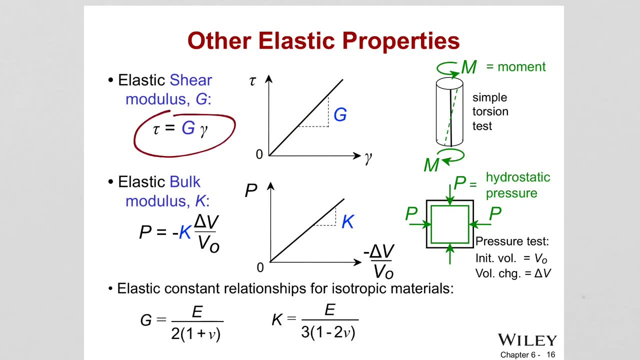 0.5 and 0.5. this is, as i explained, is the shear modulus and this is obtained from the shear stress versus shear strain curve and with the torsion test, and this g is again the proportionality constant between shear stress and shear strain. there is also one more modulus: 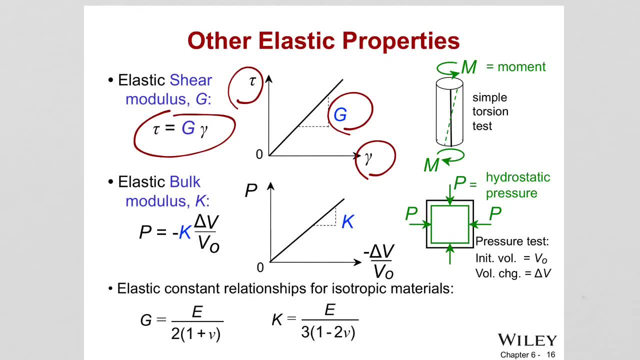 and this is the modulus we called bulk, modulus k, and this is when the part is exposed to hydrostatic pressure in all axis, it is under compression and in this case p is the applied stresses again and the deformation, the strain is. overall volume is changing right. so 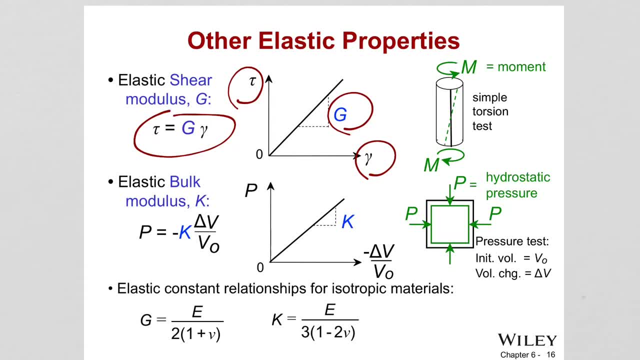 delta v over v0, the volume. delta v change in the volume over the original volume and if you record this change for a part that is under hydrostatic pressure, the slope is going to give you k, so it's the bulk modulus. all these modulus volumes depend on atomic bonding strength and all these are actually 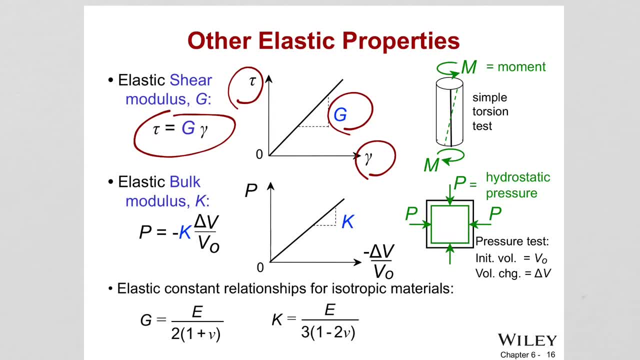 called hoops law, because it is providing us linear relationship between stress and strain and besides that, we can correlate the moduluses to each other. so if you want to figure out one modulus and but you know the other one, you can use the equations that correlate those moduluses, such as: we can find from e what is the g. from e we can find what: 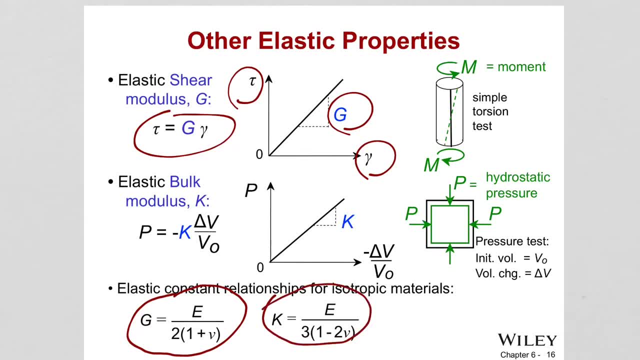 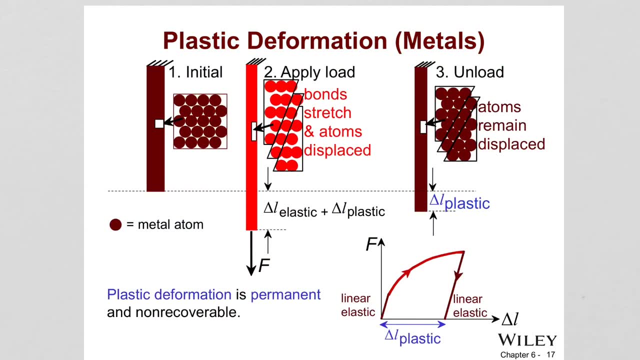 is the k to be able to do that, but you need the poisons ratio. so based on these two estimation, we can give you what is elastic deformation. when we have elastic deformation, solid deformation, or in other words said velocity deformation, so we can explosive deformation, we can feel transformation. okay, so plastic deformation. 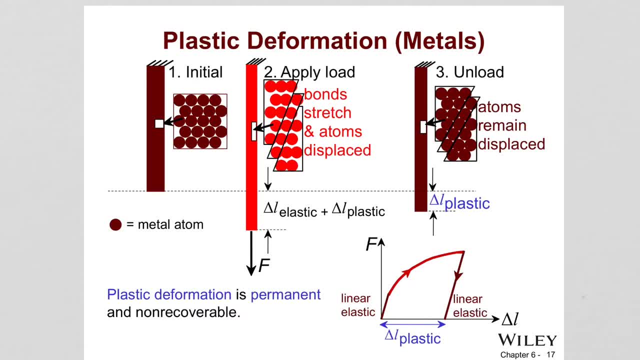 the dy 옥. you can feel it is constant, escola. we can feel it is constant. so, elastic deformation: if it is elastic And when we apply the load, what happens is first it is elastically deformed, then there is permanent change in the atoms will slide over each other, Atomic layers will slide over each other. 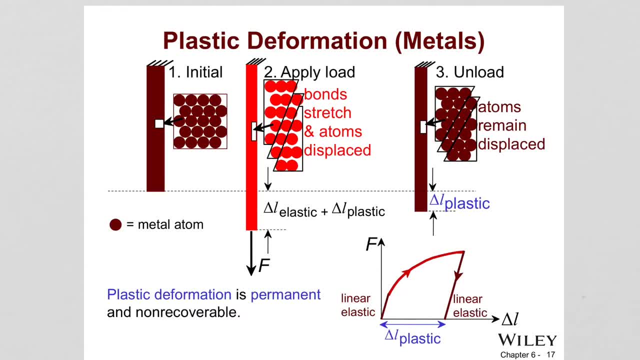 And this is going to be the plastic part of the deformation And when you unload it you will recover the elastic portion, but there is going to be some plastic deformation is going to remain. So the part is elongated. You cannot go back to its original shape. in number three, You see, when you unload it, still a deformation remains and it is called plastic. 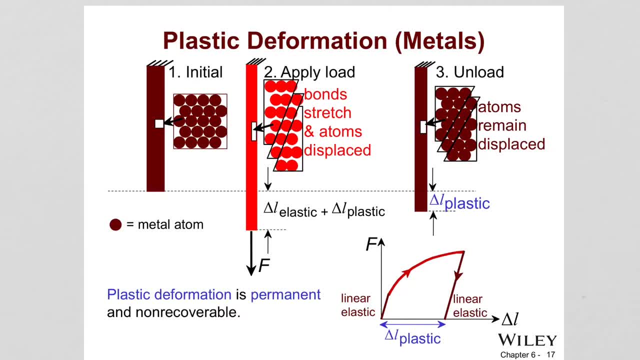 So plastic deformation is, as I said, permanent and non-recoverable, Right. So you can see here the force and this change in shape. You can see the linear elastic region here, And then the plastic is nonlinear. You see now how force and change in the length is related. It's not a linear relationship. 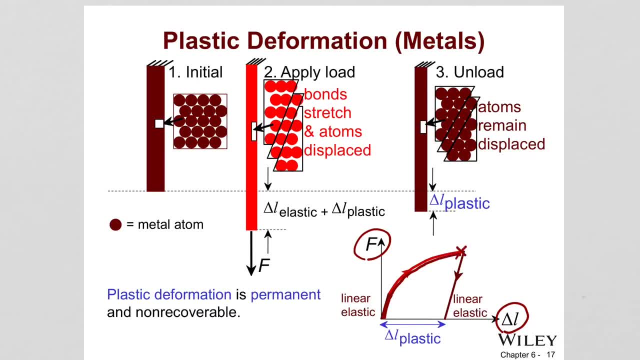 It's nonlinear And at some point when you remove the stress, you go back to a deformation which is remains in the structure. And this much delta L remain in the structure, But this part recovered, The elastic part, the linear elastic part is recovered. 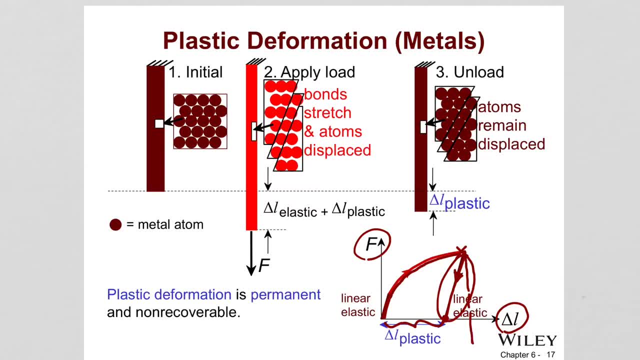 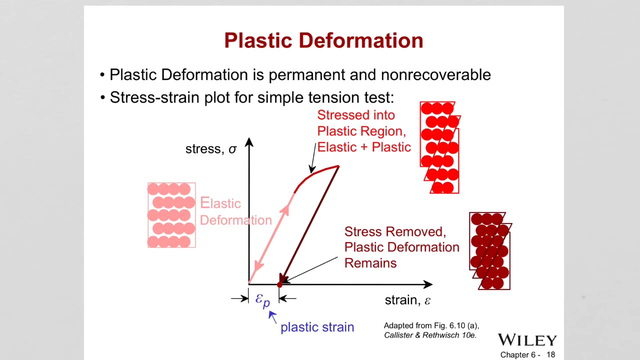 So normally your deformation is this much. But this much is recovered OK and this much is removed. The delta L plastic is remained in the structure, So this is called plastic or permanent deformation. This again summarizes the stress strain curve K, So the. again the machine records the force and change in length. 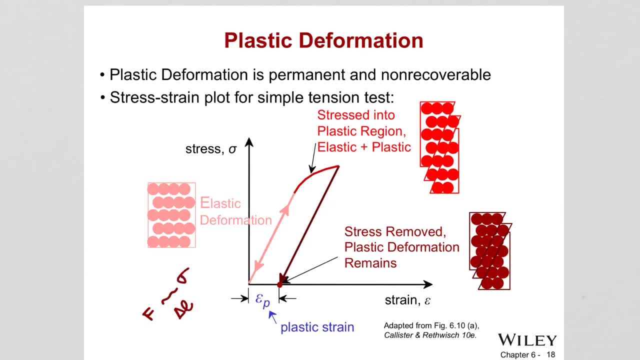 And converts them to state Yeah, Yeah, OK, stress, using the equations we learned, and strain and then gives us stress strain curve. it measures the force that needs to apply to keep the deformation rate constant and then gives us the stress strain curve and in elastic region it is recoverable because it's just 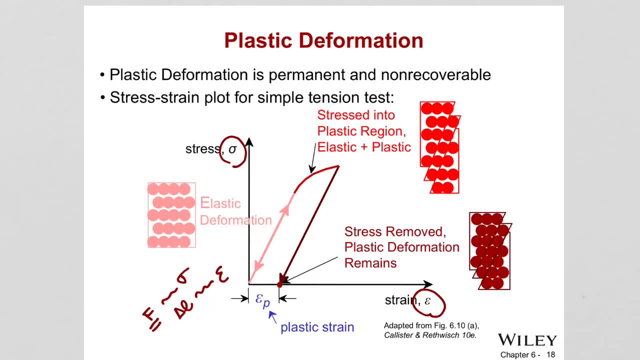 we are stretching the bonds between the atoms and when we relieve the stresses, it go back to its original position. right, it goes back, but after some point is reached the plastic deformation will start, meaning the layers of atoms slide over each other, and later we gonna see this. 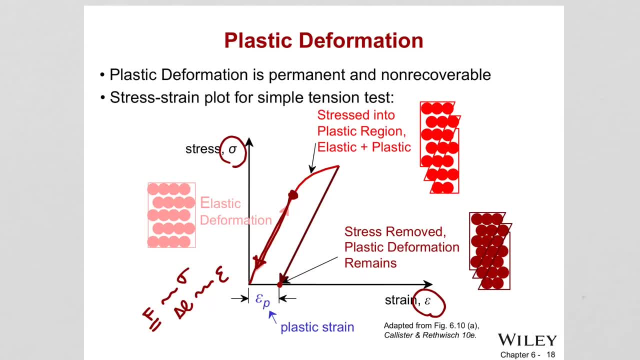 is gonna be certain atomic regions, certain atom planes. that has required the lowest amount of energy to move those who are the ones that are sliding initially over each other and dislocations are helping it. so by the motion of dislocations the material is the deforming plastically. so 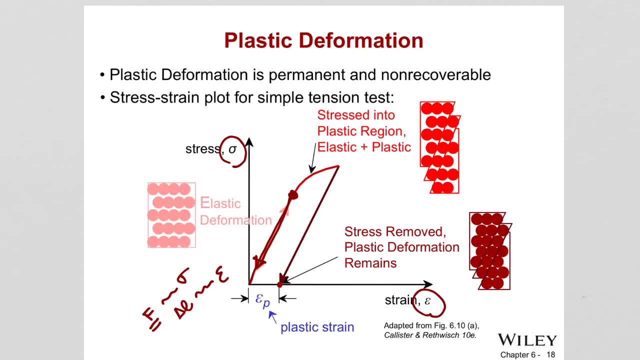 the material will keep deforming elastically, together with the plastic deformation, so there will be a region that is performing it's deformation. therefore, there will need a few acting actions, a region where there is both elastic and plastic deformation going on. so, from a non, from a linear 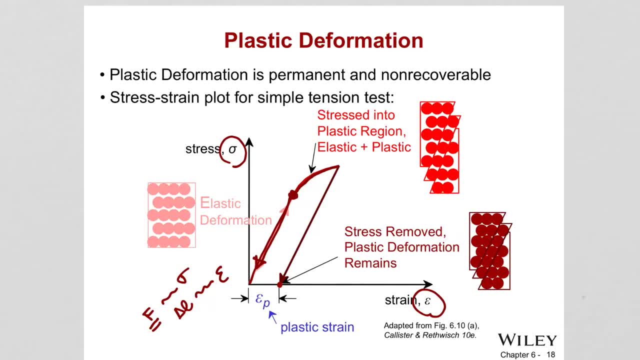 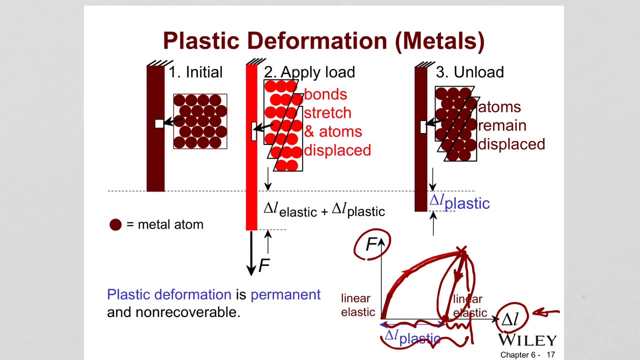 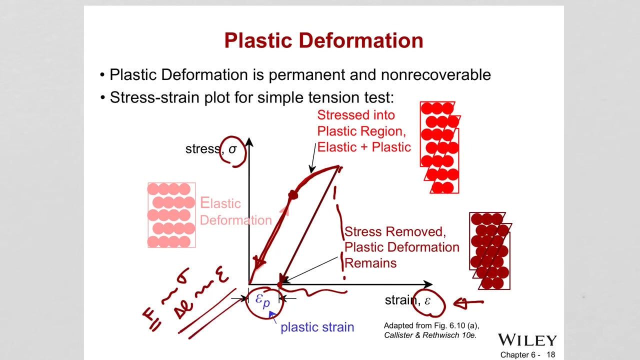 region, we go to a nonlinear region and when we remove the stress, we recover some. we recover some elastic and plastic strain remains. so this is just, this is what the data is collected, but this is the water the equipment gives us converts to stress, to strain, using the relationships we 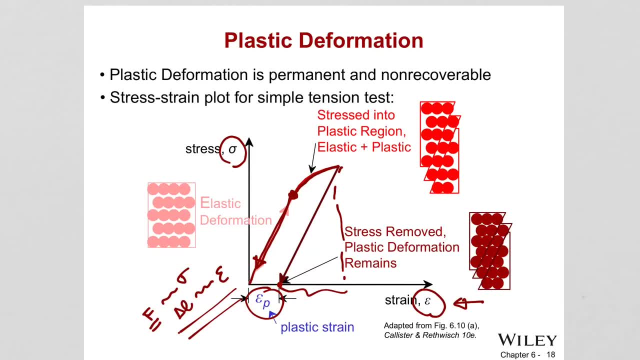 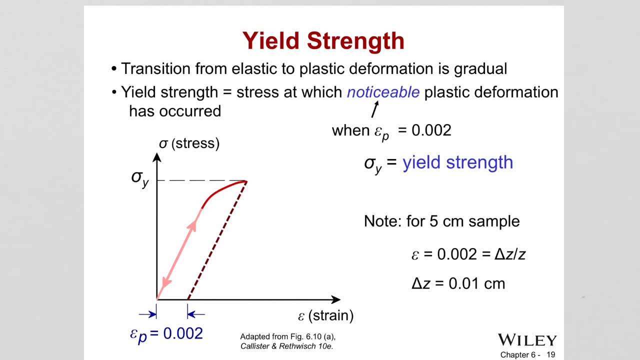 learn. so when there is a transition from elastic to plastic deformation, this can happen in some materials like aluminum, gradually. it is dangerous, except some of the materials you can use. but when it is a transition from elastic to plastic deformation to elastic deformation you can cannot be an obvious change from sudden elastic to plastic and there has to be a way to figure out. 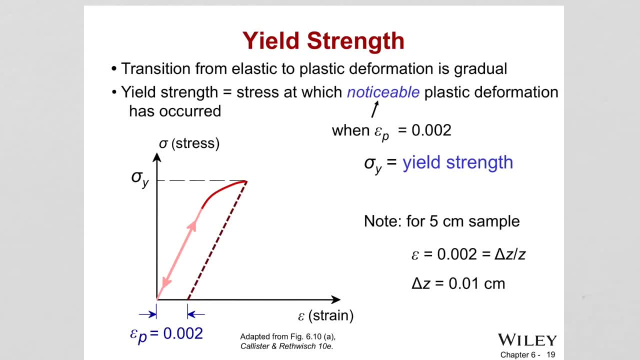 from the stress strain curve to determine the yield strength of the material. Yield strength is basically the stress where the plastic deformation noticeably starts And in design you never want to go over the yield strength of a material because whenever you go over the stress values, that is exceeding the yield strength of the material. basically the part is gonna go. 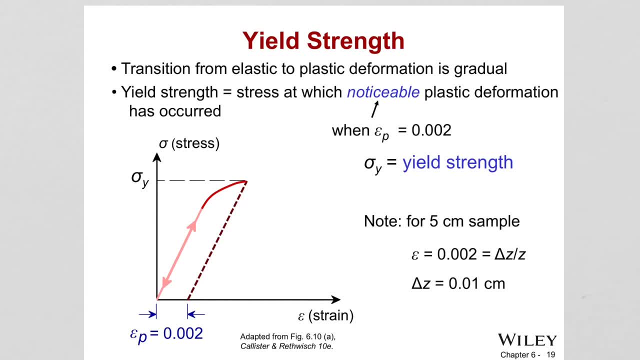 undergo plastic deformation and then, basically, material fails to serve us its purpose. So, to get an information about what is the yield strength from the stress strain curve, first of all, that is defined with a sigma y, which is the yield strength which we choose, a deformation amount which is 0.002, okay, So choosing for allfor all cases. 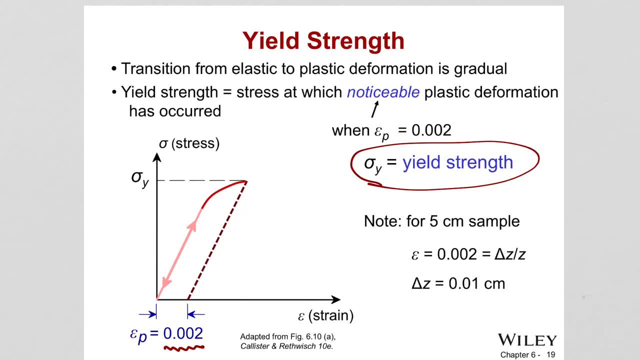 basically, for all materials we choose the standard strain amount of 0.002 and draw a parallel, the linear region, like a parallel linear region, and find its intersection with the stress-strain curve and then go to the y-axis to read the yield strength. 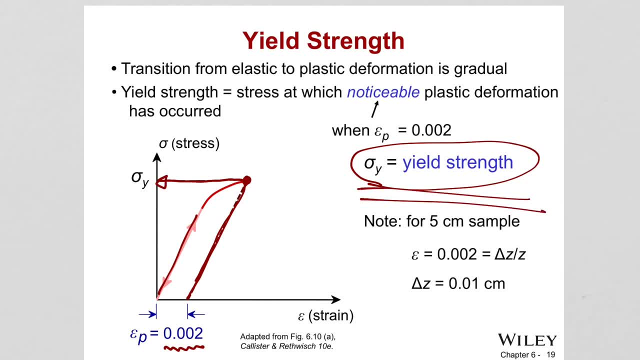 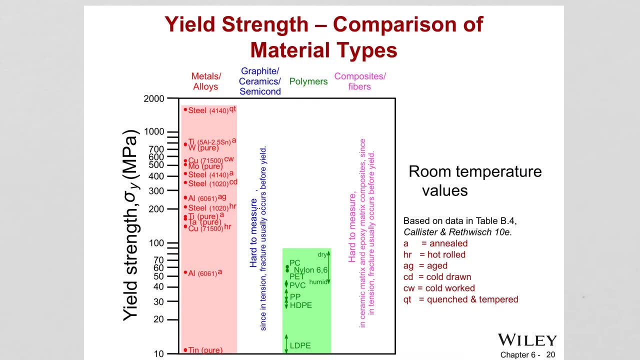 okay this, we do it for all materials, so we have a standard way of reading. what is the yield strength? when we compare the yield strength of materials- and this is gonna be for metals- against ceramics, graphite polymers, composites, so for metals and alloys we are seeing steel has a very high temperature. 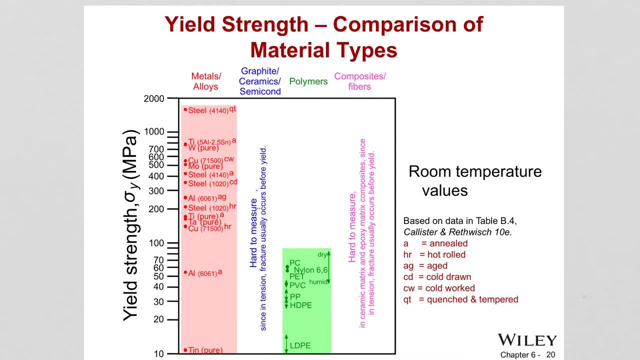 of course these are different type of alloys. these alloys can go through different type of heat treatments. for example, qT means for steel, quench and tempered. So later we're gonna learn these heat treatments, because sometimes materials, to enhance their properties has to go through certain heat treatments, meaning we increase the temperature than 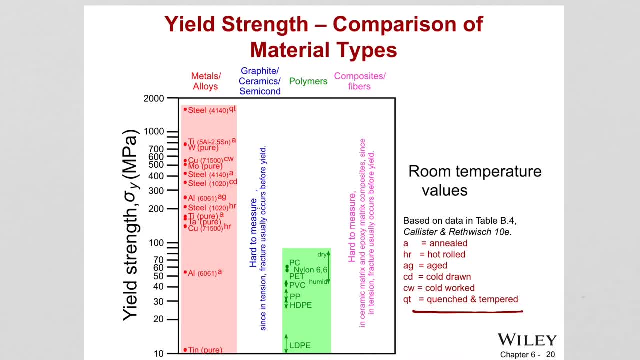 senos bye, suddenly quench meaning. quench meaning suddenly drop into water, and this causes, for example, small grains in steel. therefore, the strength of the material is increasing, for example, or different type of heat treatments can be given, depending on these letters we are seeing. okay, and then right? 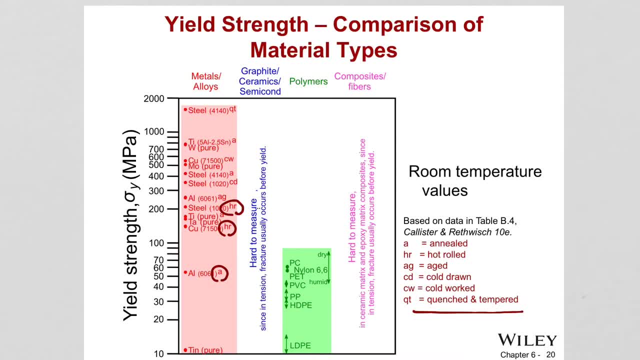 now you don't worry about these, because later we're gonna see how deform a how heat treatments can affect the strength of the material and basically this is changing. these treatments are changing the microstructure, grain size and therefore, of course, changing the interaction of this grains with the dislocations and therefore changing the strength of the material. you don't. 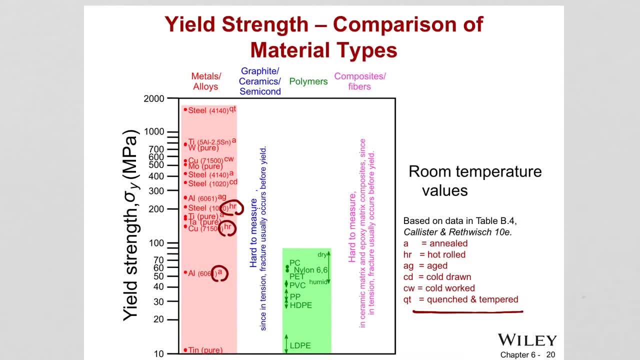 have to worry about that part right now. we are just comparing the yield strength of materials with within each other. so the ceramics had are hard to measure because they intentions they are not strong. okay, they are stronger under compression. the very reason for that the ceramics are susceptible. 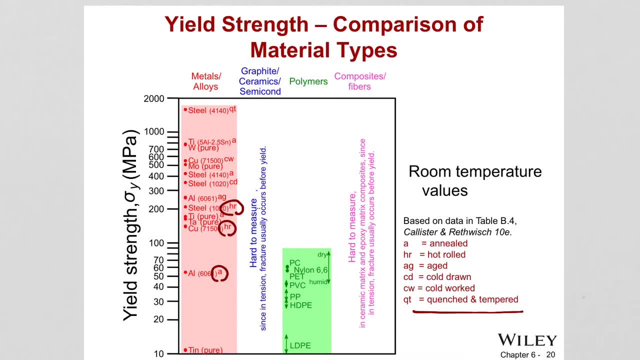 to sudden fractures and when we look at the failure chapter we're gonna see that. okay. so because ceramics usually have pores and cracks inside them and when we apply the tension this crack can propagate and then material can separate into two parts, basically suddenly fail. but under compression the crack doesn't propagate because basically you are not properly compressed, you are 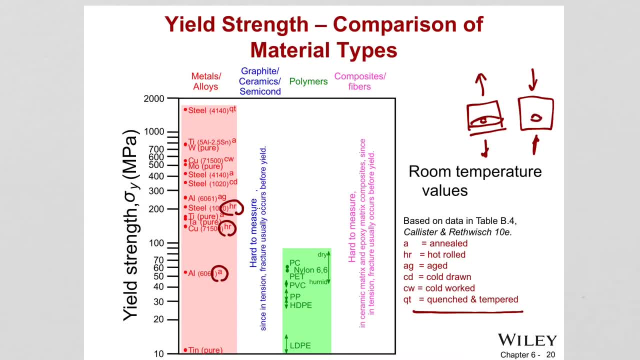 cooling the crack apart, right. so that's why these materials are very good at under compression. polymers have low strength values because the in weak intra molecular bonds, composites and fibers. this is also um hard to measure because, uh again, the fracture can occur before the yield. so 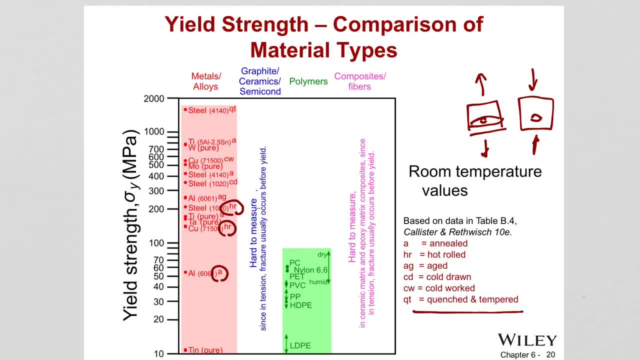 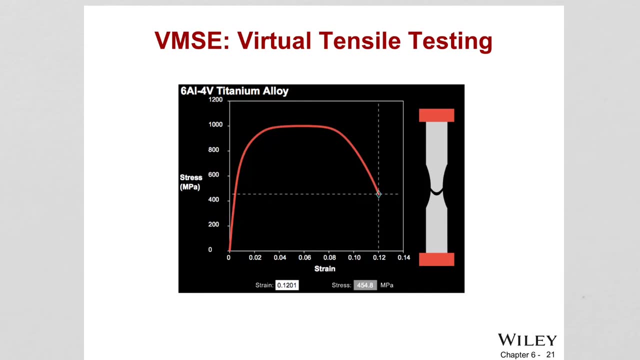 we can only make logical comparison between metals and polymers and we know metals are strong compared to polymers. so this is some data from virtual material science and engineering. i provided you to link and go to that link and, depending on the alloy you choose, it will give you the. it's like a simulation. 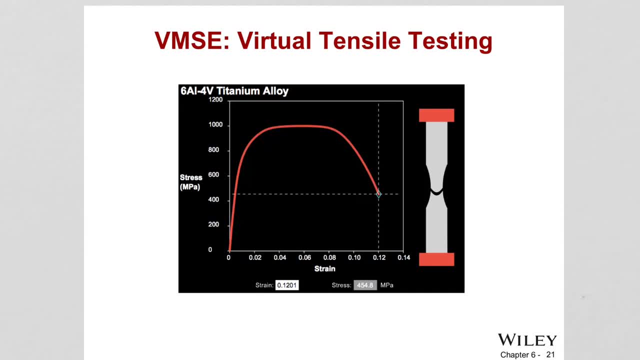 of how this process works and then you can choose your material size and pre-есь back to the original stress strain data is collected and on the right you can see how the how the material is changing in dimensions, depending on where you are at the stress strain curve. so I would suggest you guys to go to the link that I gave you and 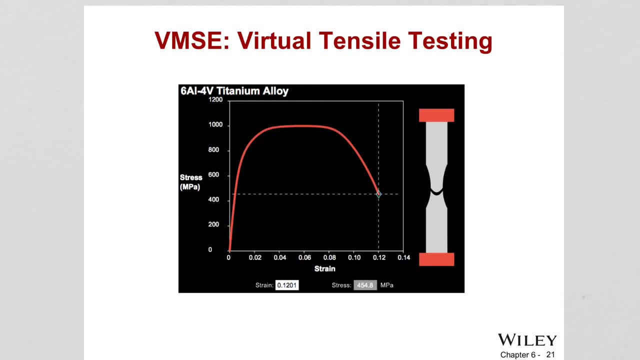 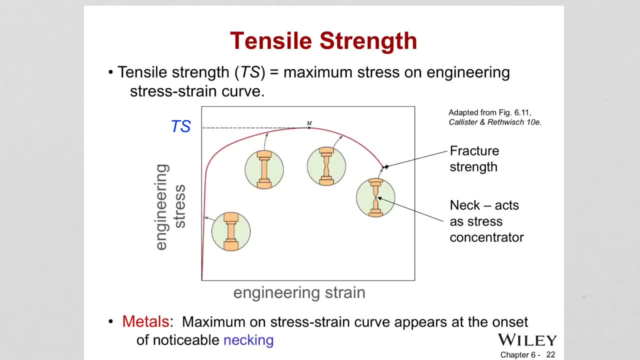 then observe some of these strain strain stress curves for different materials. so we learned about yield strength- right, it was the transition from the elastic to plastic deformation. and now we're going to learn about tensile strength, sometimes called ultimate tensile strength, and that is the maximum stress. 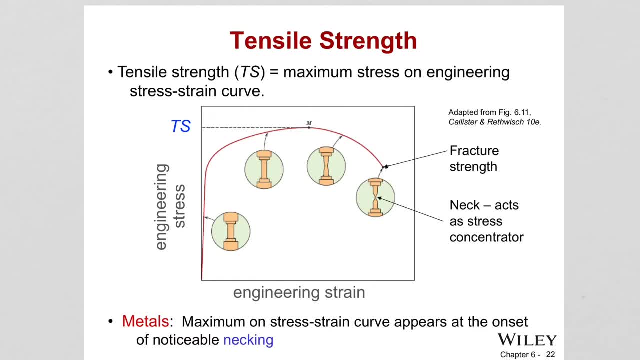 on engineering stress strain curve. so the stress strain curve we have learned so far that is called engineering stress strain curve, because the force in force data is divided to original cross sectional area. but in reality the cross-sectional area is changing throughout the test. but that doesn't include that information. 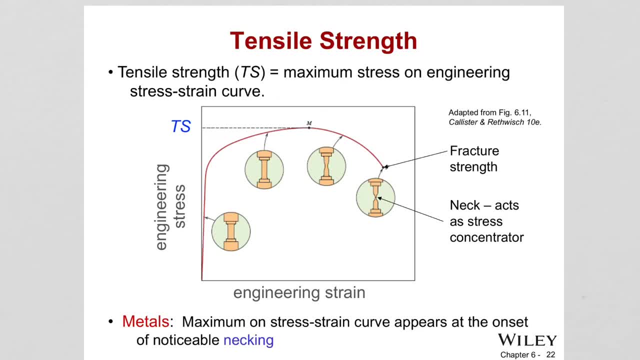 ok. so initially we start with application of the forces And then material elongates. This is elastic region. We go to plastic region now, which is nonlinear. The material starts to deform permanently And at some point you reach a maximum. This maximum is where we read the tensile strength. 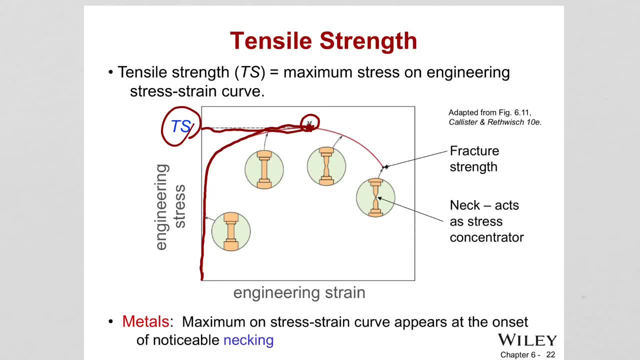 And then, at certain point, when you reach that maximum, there is the thing called necking happens. That means the cross-sectional area of your specimen is now getting smaller. Okay, Since now the cross-sectional area is getting smaller, the device has to apply less force. 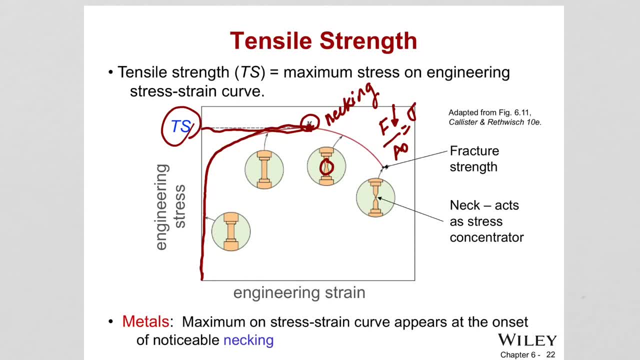 To achieve the same deformation rate. Remember, the device has to keep the deformation rate constant. But since it needs to apply less forces now because the cross-sectional area is lowering, what happens when you put it into the engineering stress definition equation? it was forced over original cross-sectional area. Since force is lowering because the device needs to apply less force now. 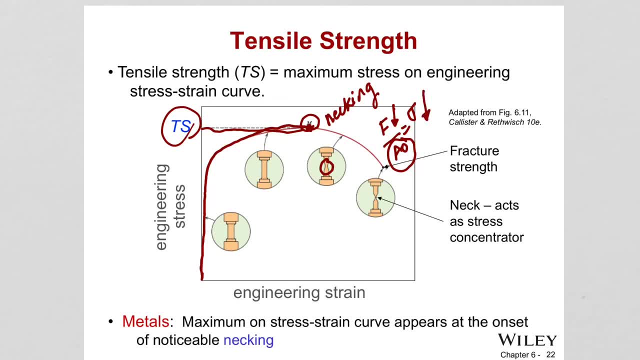 the stress is also lowering. So that's why we see when the necking starts we see a decrease in the stress. Okay, Until certain point. at certain deformation strain the material breaks. So we call that point is fracture strength? Okay. 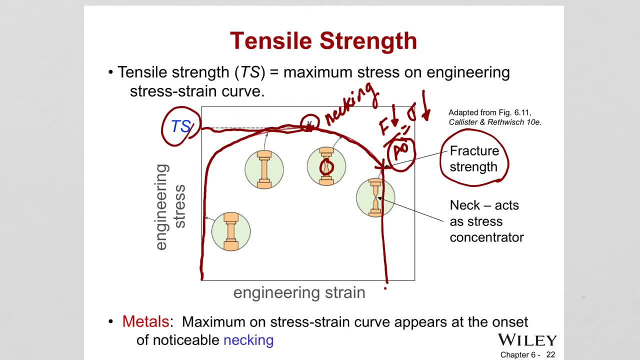 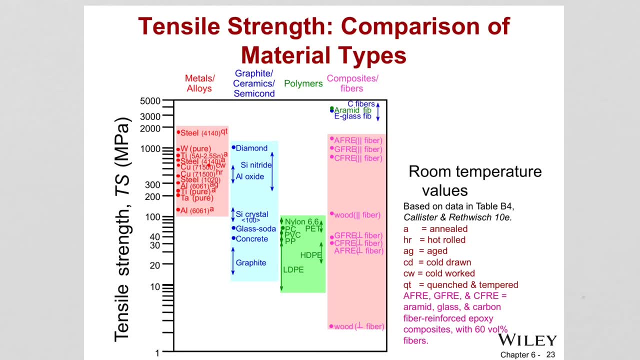 All right. This table again compares tensile strength. So if you look at the stress-strength curve of each of these materials and choose the maximum point it reaches and then read the strength volume from the y-axis, that is going to give you the tensile strength. 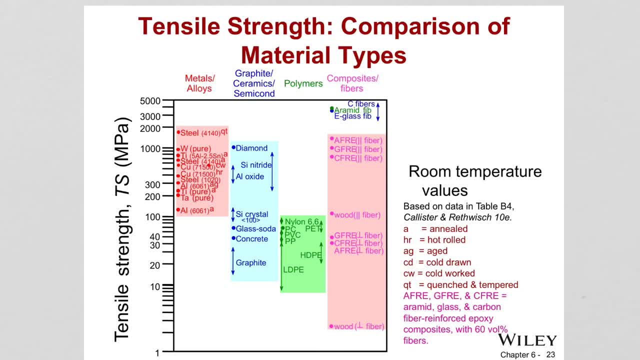 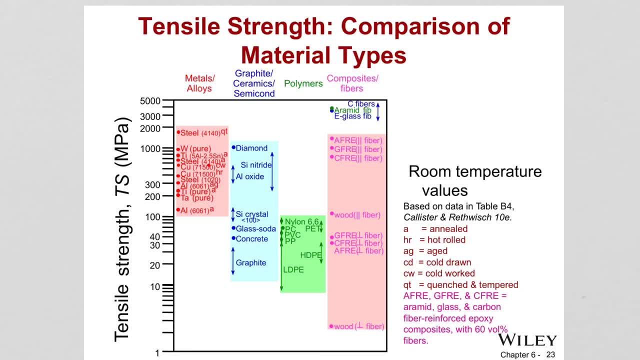 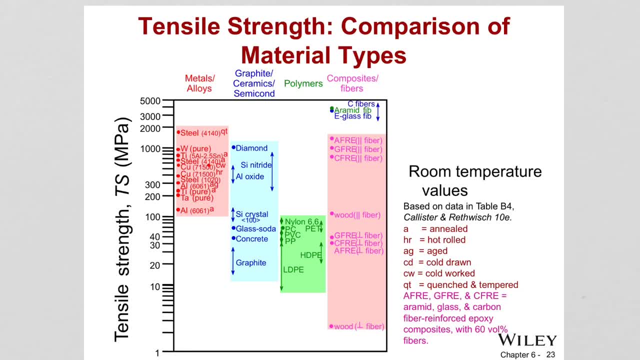 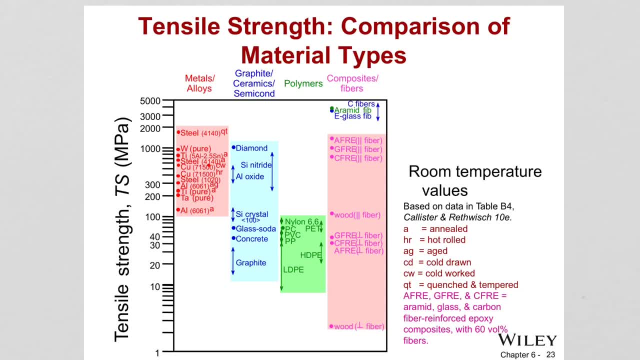 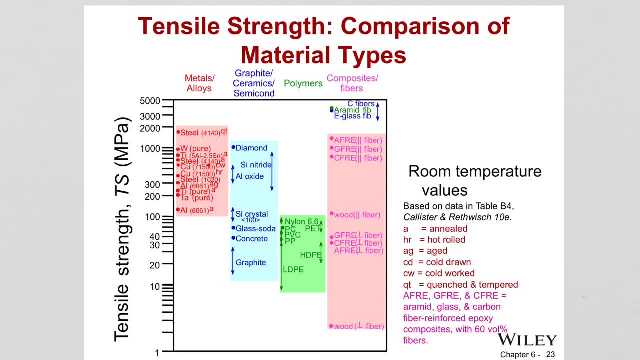 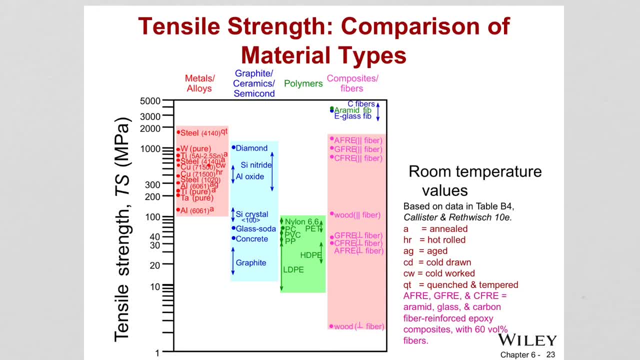 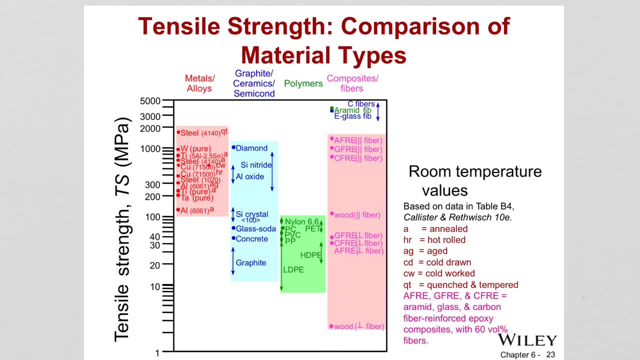 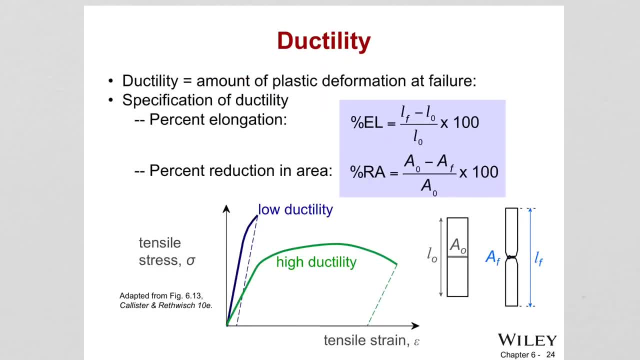 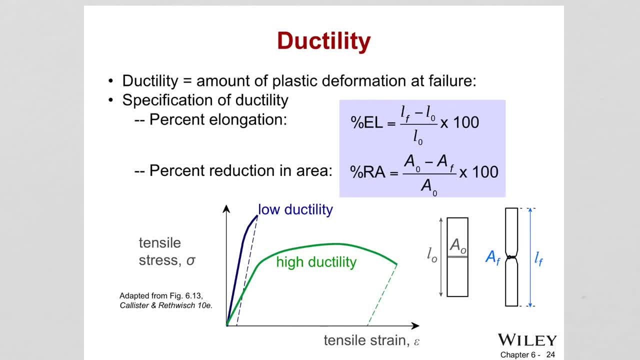 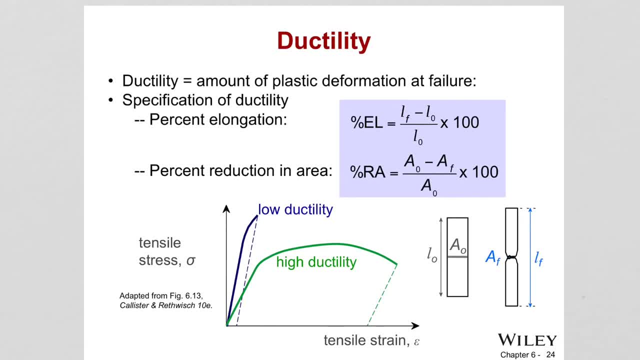 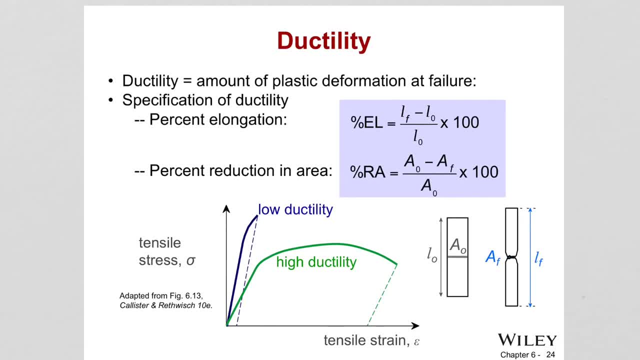 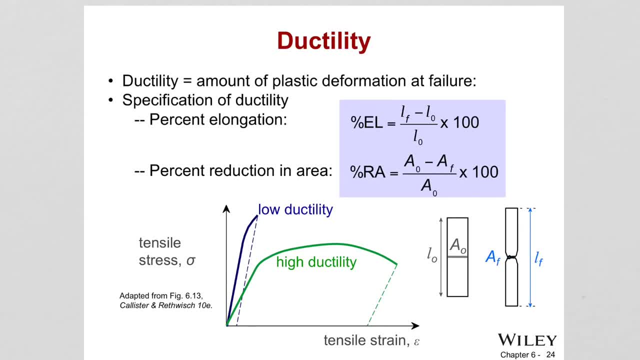 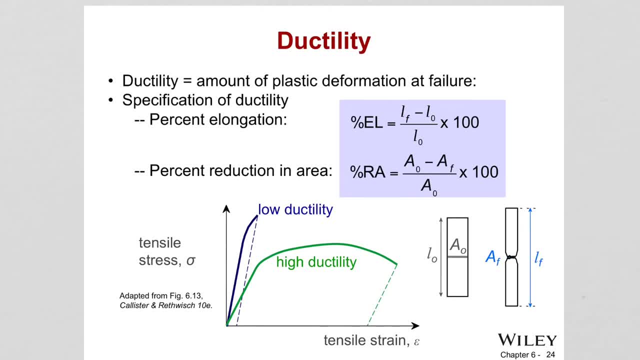 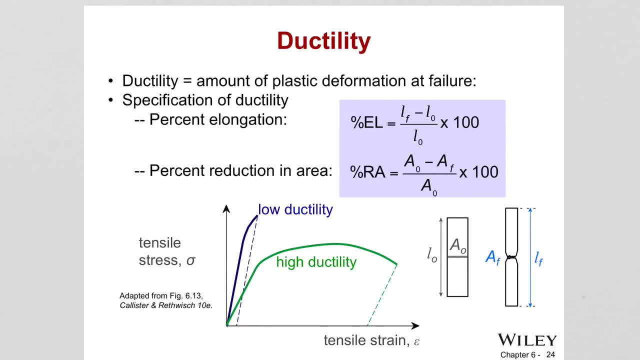 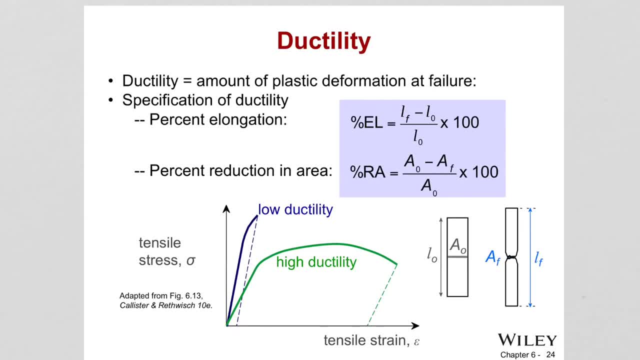 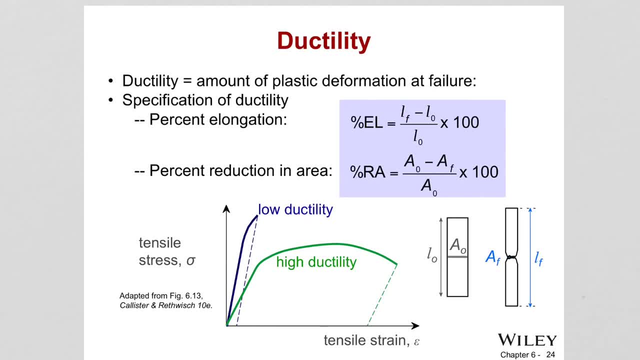 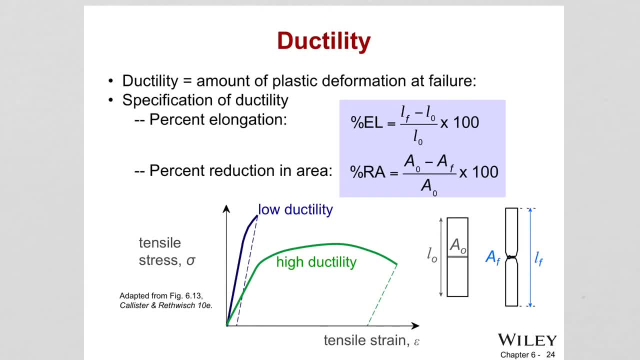 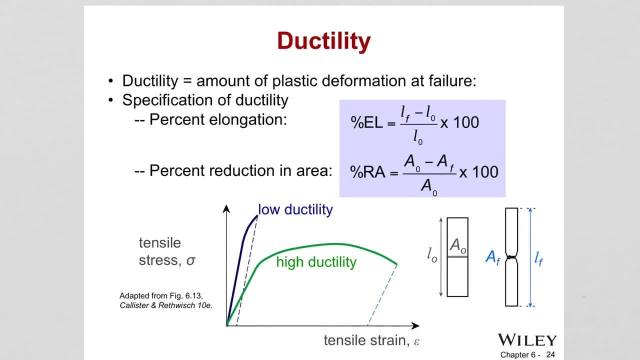 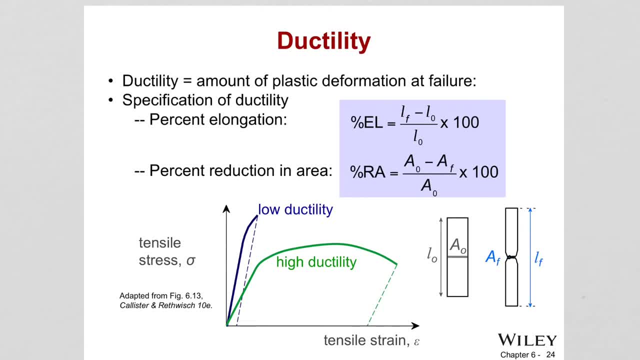 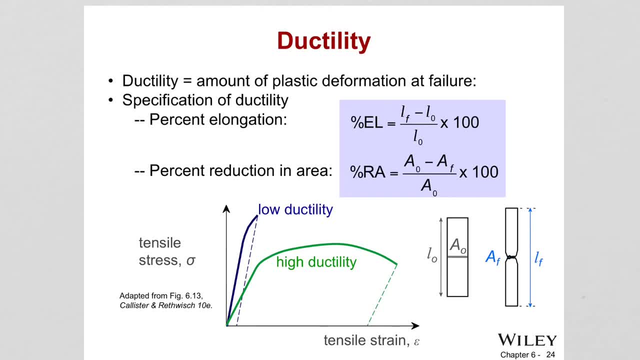 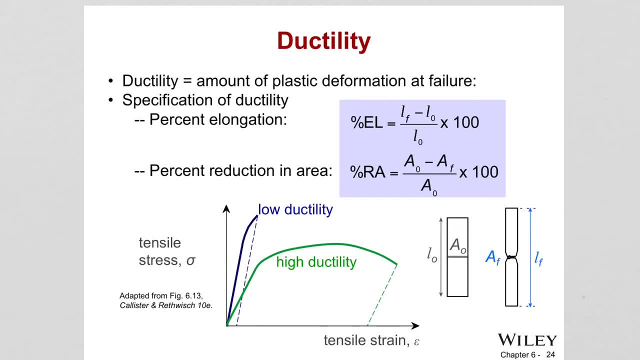 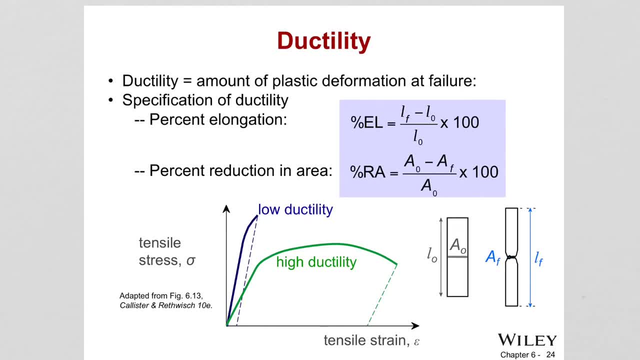 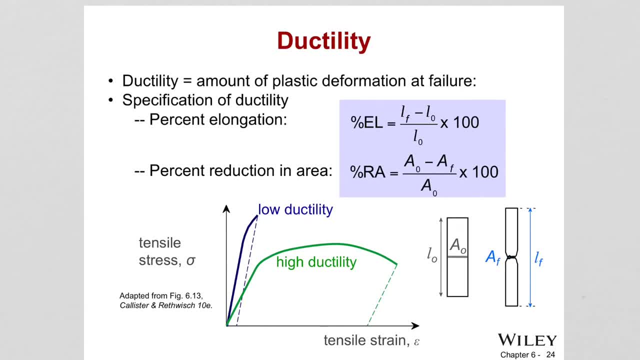 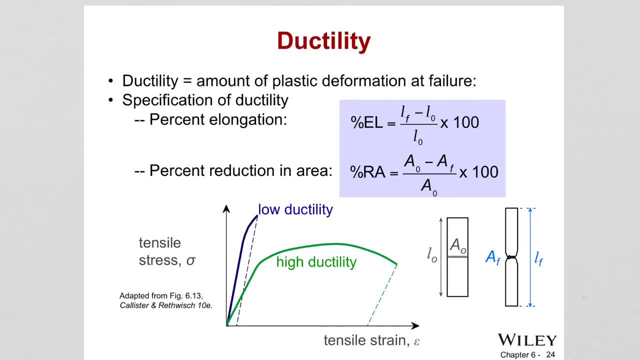 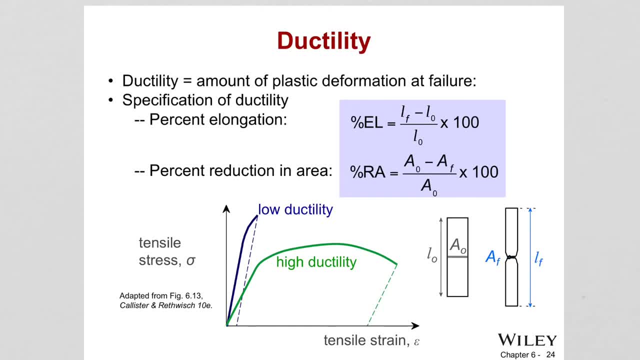 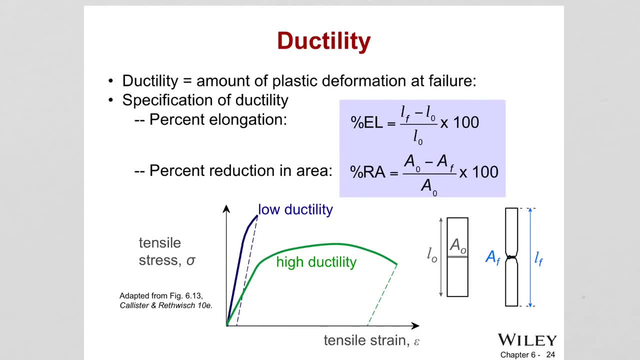 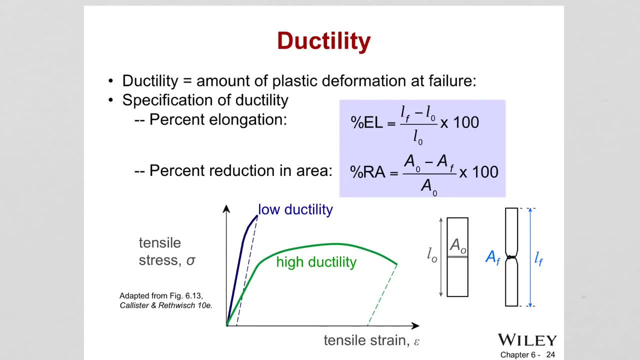 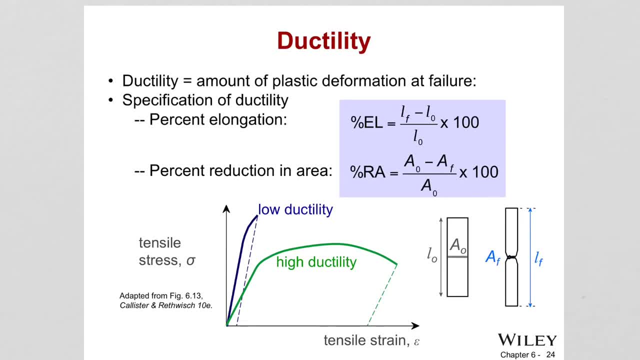 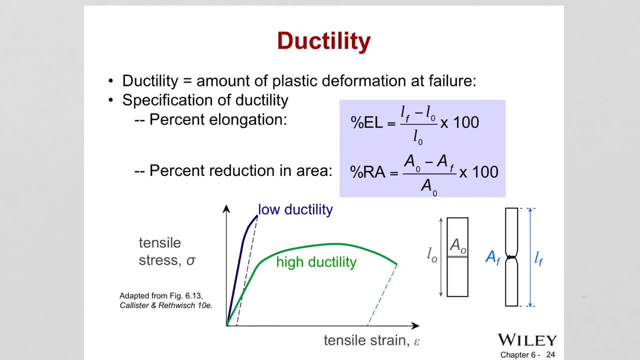 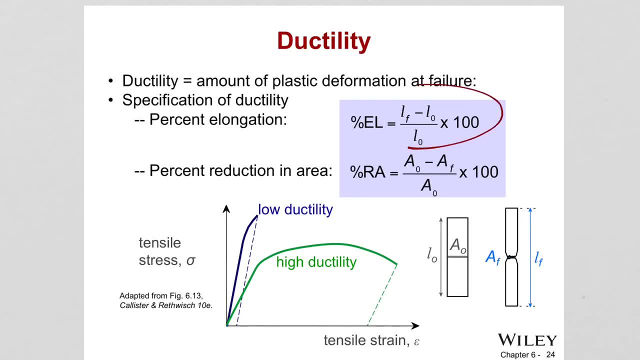 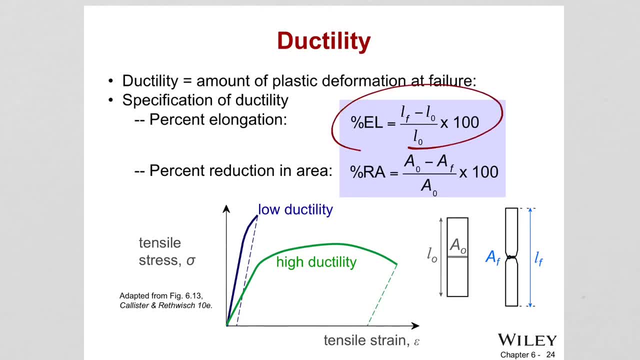 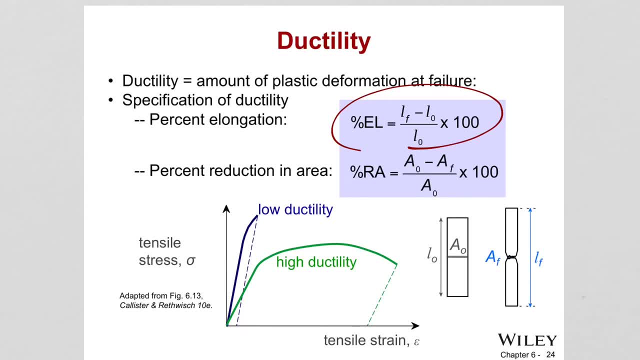 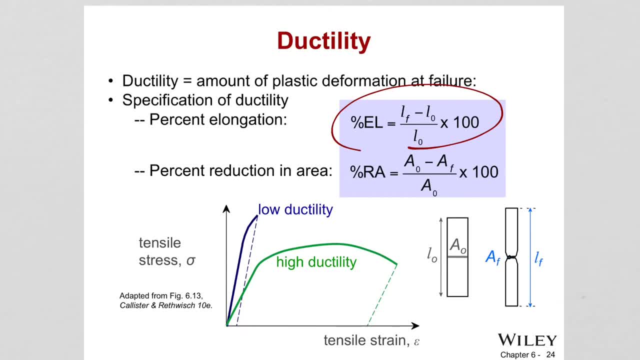 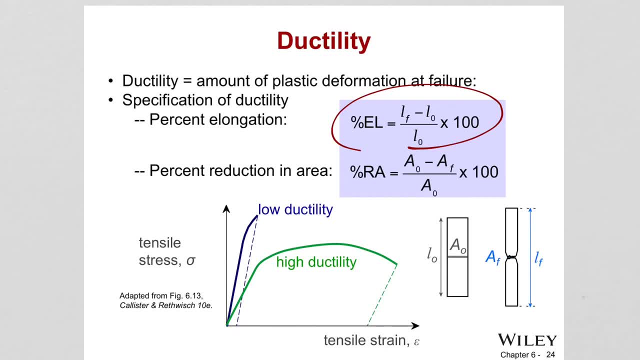 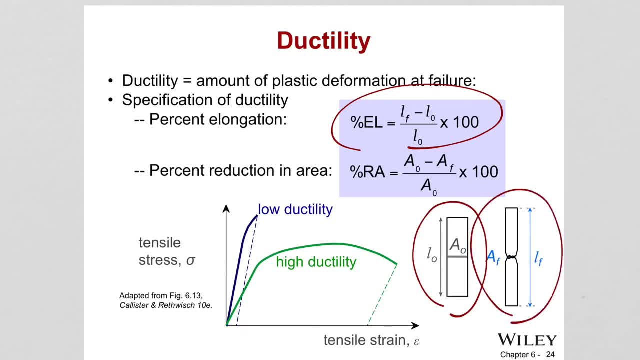 than the final cross-sectional area Over original cross-sectional area. times hundred is the percent reduction in the area. Both gives you idea about the ductility of material. You guys need to understand. what I can ask in the exam is I can give you stress strain curves of different material and I can tell you to. 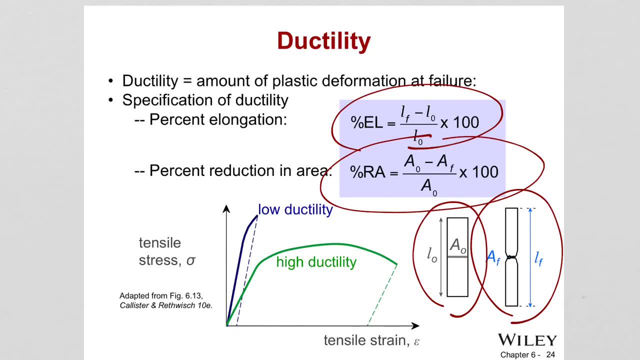 compare them like which is more ductile, which is more brittle, etc. So when you have low ductility, it's brittle because it immediately fractures after some strain, and some materials have high ductility, you can see it deforms to a large extent. Okay, so of course this is the plastic deformation, so it doesn't. 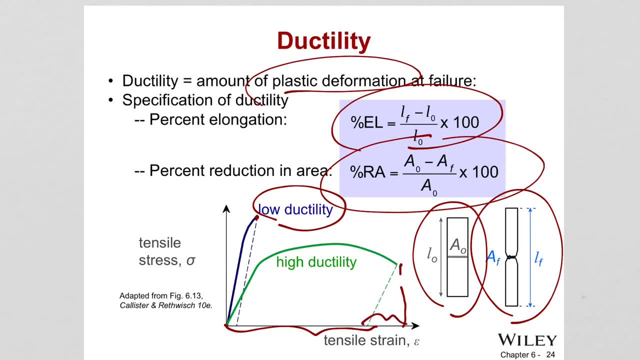 include ductility, Elastic recovery here. All right. anyways, from looking at the x-axis and seeing how much it is strained, how much it is deformed, you can comment on looking at the stress strain curves. what is the ductility? is it high, is it low? 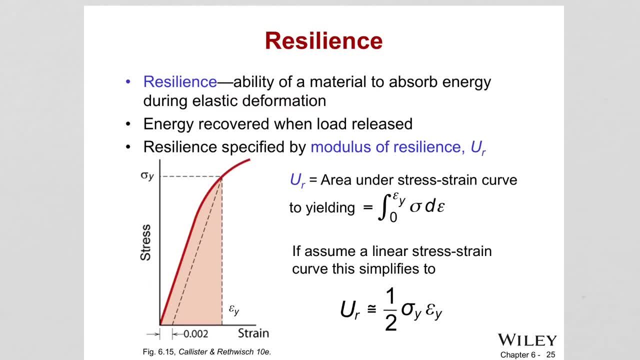 Resilience is the materials ability to absorb elastic energy. Think about you. are you want to store elastic energy in the material? Okay, so think about it's a spring, you are stretching it and as you stretched, you are doing work on the material, because force times distance, right, these material, these bones are. 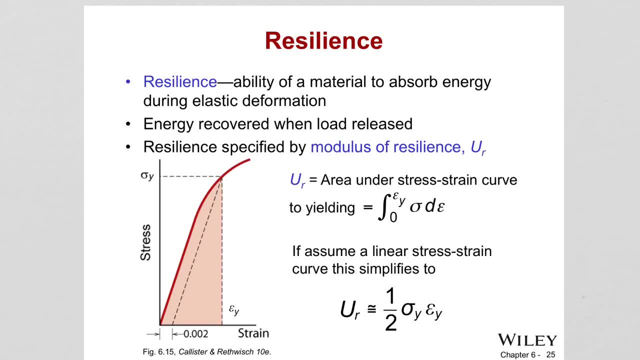 with applied force, they are stretched. so force, time, distance is work. Work is energy. Basically, by stretching the material, you are storing energy inside those bones, those springs in between atoms, basically imaginary springs, That energy is recovered when we release the load. Okay, so what is resilience then, if? how we measure it? if 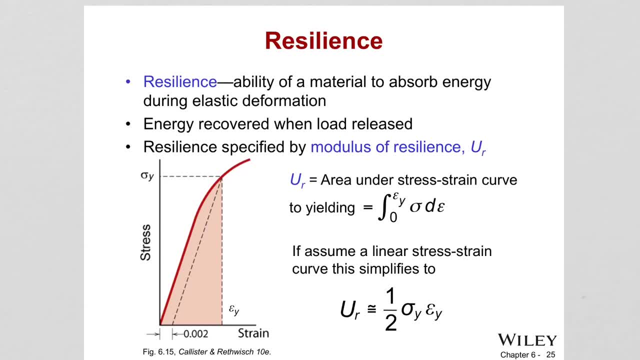 we look at this under the stress strain curve and find the yield strength and from the interaction of the yield strength line with the curve, the intersection of that line, you go down and find the yield strain Okay and that region is going to give you the energy absorbed within the material You can. 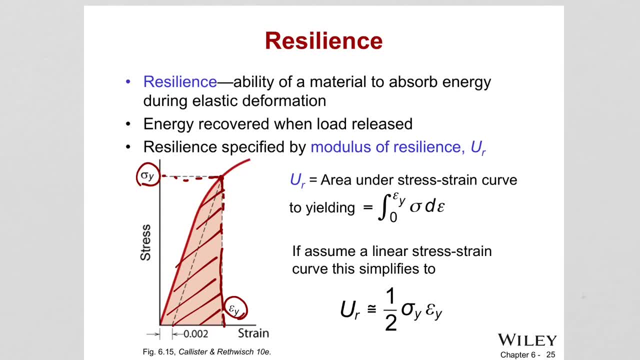 compare these areas of different stress strain curves and then comment: this area is bigger in that material. that means it absorbs more energy. This energy, or resilience, is shown by modulus of resilience U with a subscript R. This is the area under stress strain curve until yielding. So what does that mean from? 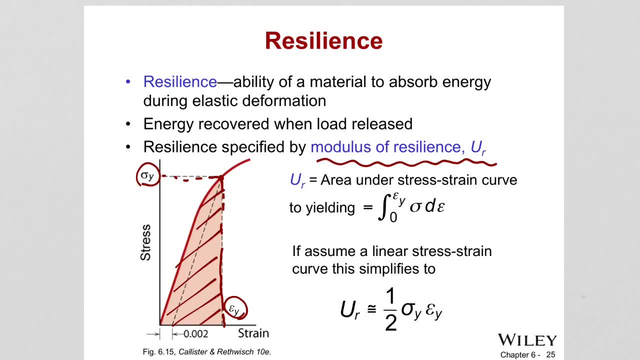 So area means integration, right From zero to yield strain, integrate, stress strain curve, strain curve. okay. So with infinitesimal changes of the yield strain, just integrate. take the sum up of all those little interactions, basically, Okay, so it will give you this equation. integral means the area right, So it will give you the area under the stress strain curve. If you assume it's completely linear change, okay, it's completely linear. here that means it's a triangle. 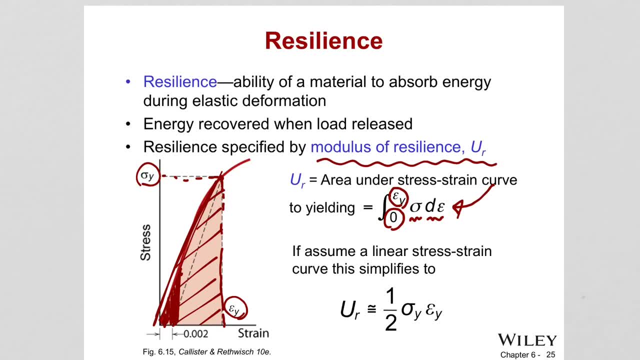 So actually, if you want to find the area, you don't have to go through this integral. you can say it's an area of a triangle. So what I do: multiply yx, Yx to the x-axis, and divide into two, It's like area of a triangle. you can simplify it too. 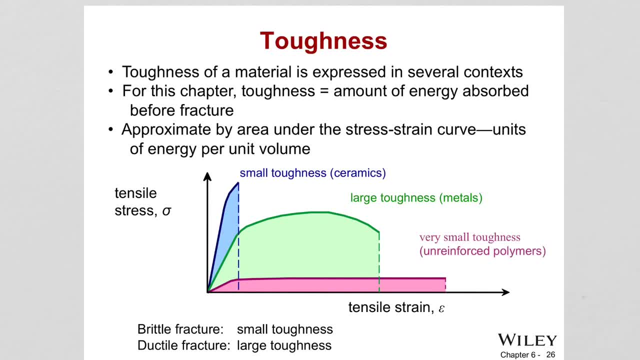 What is toughness- So resilience- was energy absorption till elastic within the elastic deformation region. Toughness is energy absorbed till fracture, So it includes all the all the areas under the stress strain curve. okay, By definition it is giving us units of energy per unit volume. So we look at, if we try to compare, the blue one is small toughness because the blue area is smaller compared to the green curve where the area under it is very large. 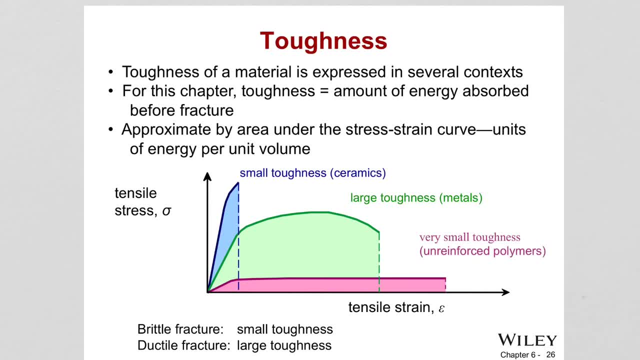 But the pink one is also: even though it's very ductile it has small area, meaning its energy absorption is small. brittle materials have small toughnesses and it fractures immediately here. but the fracture it takes for this one to experience it takes a long deformation, long energy absorption. So the ductile materials are generally have large toughness volumes. So you can correlate between 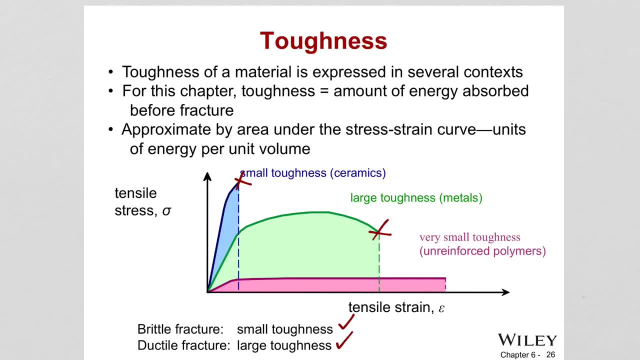 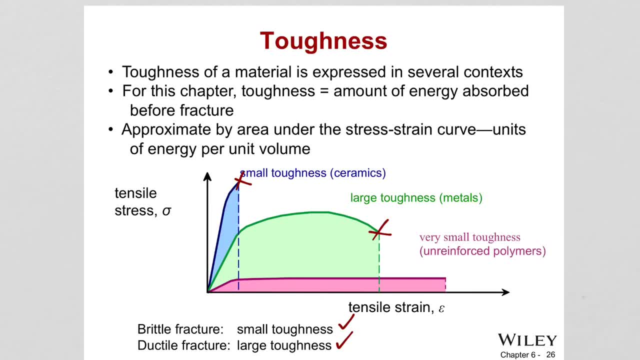 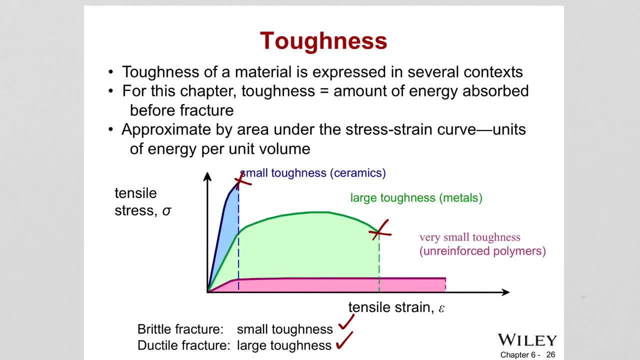 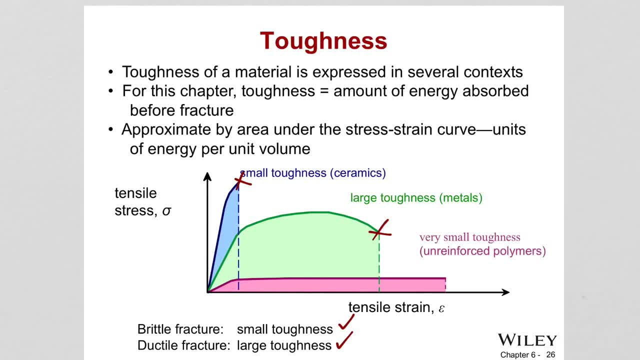 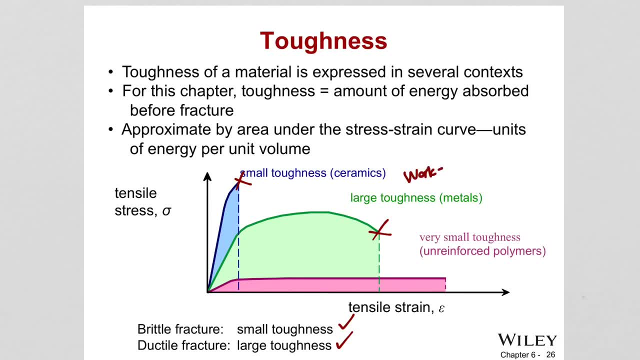 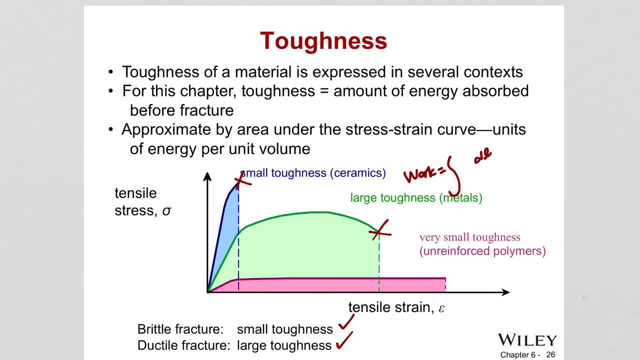 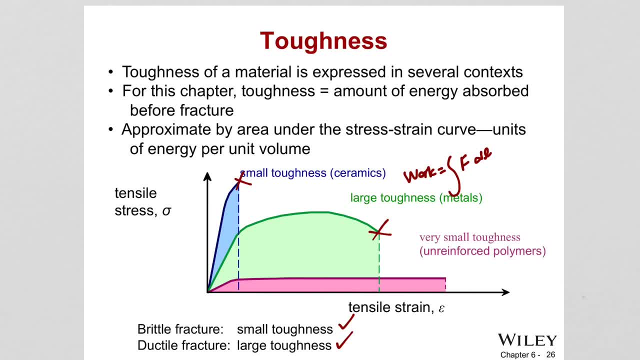 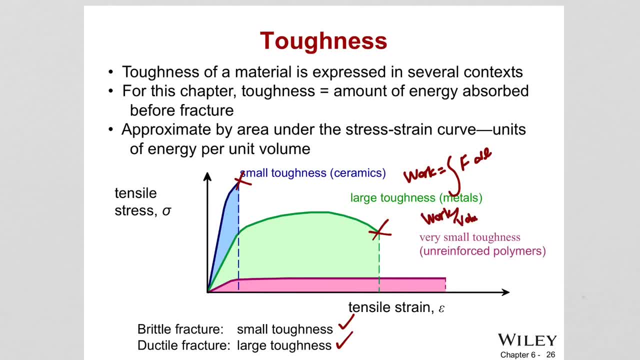 ductile and brittle materials to how much energy they will absorb. right, we gonna divide then to volume, which is area times length, and this will tell you: force over area is stress, the L over L is the deformation strain. so therefore, by definition, the energy absorbed per volume is the area under stress-strain curve, and this is giving us the toughness, the 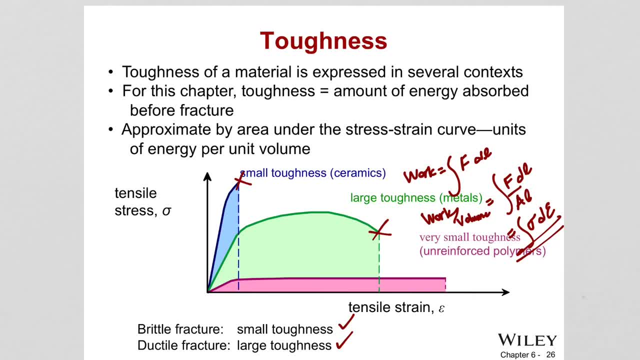 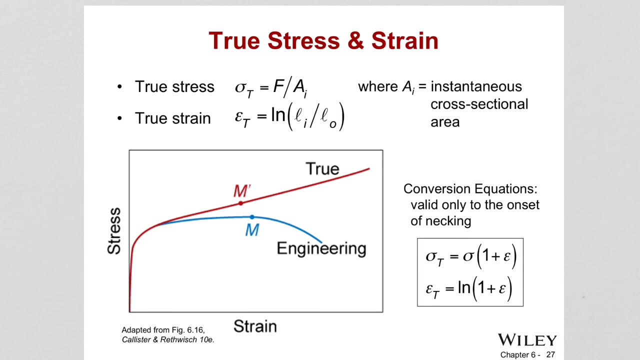 energy, of absorption capability of a material, and in some application you want the material too tough, you want, you, don't. we want to absorb as much as energy possible before it fails, such as a car bumper, for example. right, it should absorb all the impact energy. now I told you there is so far we have learned, engineering stress. 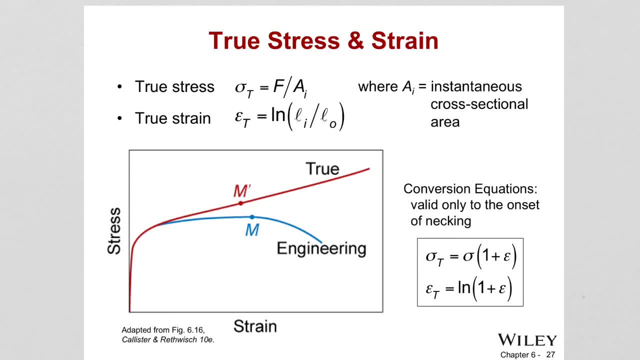 train curve because I told you, the engineering stress train curve uses original cross-sectional area to calculate the strain stress in the diagram. that's why it is decreasing, because when the force is shared between the two sources, then the remaining force is all absorbed and so is decreasing. the area is the same, the stress is decreasing in the curve. however, in reality, 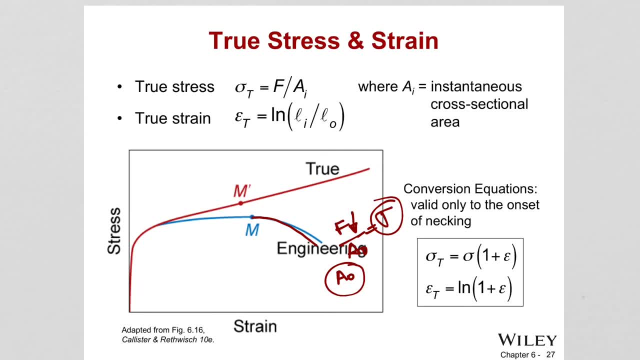 in reality it is always increasing because the area is actually not constant, like taken in this equation. it is actually decreasing too. so it is a decreasing to larger extent compared to the decrease of the force. therefore, stress is increasing actually in reality. okay, so we can see that area is changing right. it is like this, especially after this reaching: 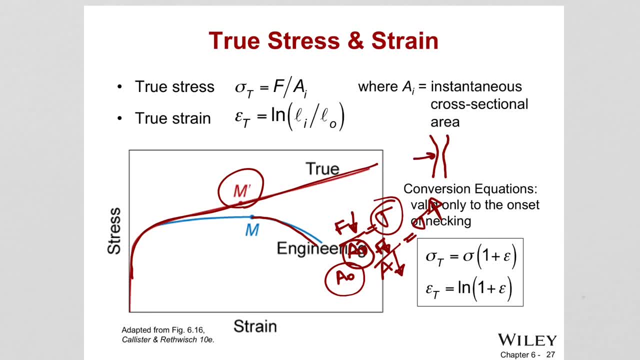 maximum where the necking starts, the area is getting smaller. so that's is called true stress strain, and equations are different. to measure this true stress, you divide it by the area of the area. you measure the area of the area of the area. you divide it by the area. 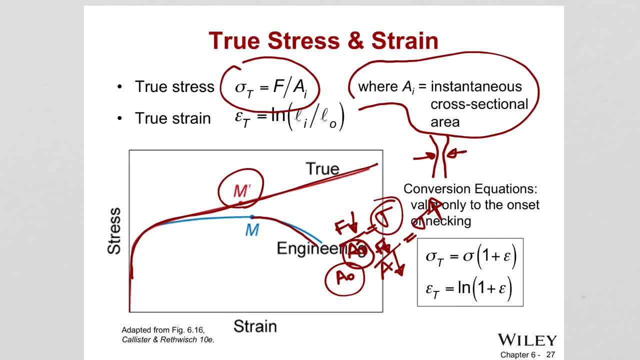 to each time the instantaneous cross-sectional area For the strain. it is given with this equation: okay, so Li is again instantaneous length. There is a relationship that relates engineering strain and stress to true stress strain and these equations are given here and these are valid only after the necking. 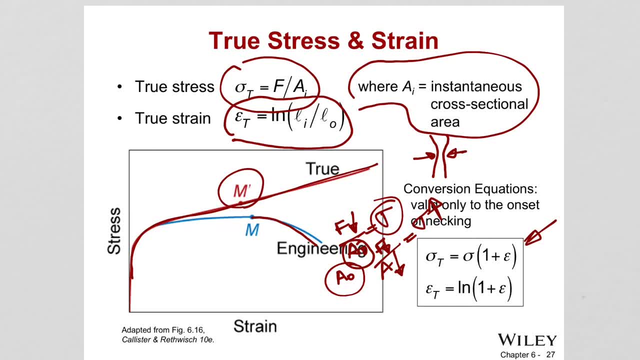 so why we don't usually collect true stress strain data is because it doesn't matter. because why? because the what matters is that the yield strength- as I told you many times in the design- yield strength or ultimate tensile strength- these are the ones that are important and up to that point, both curve. 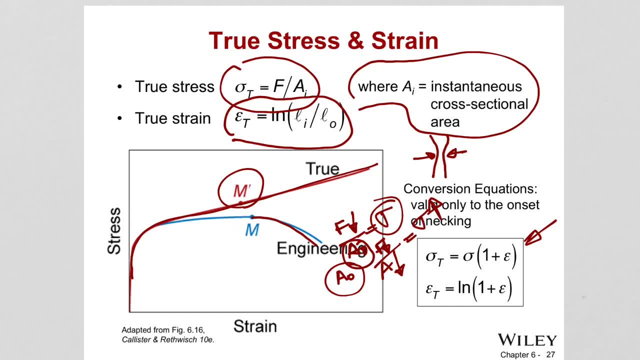 gives us a similar result, and the reason is: once the material deforms plastically, it doesn't serve us the purpose of our using it in that application. so that's why engineering stress strain curves are enough, but in reality, true stress strain curves are the real, real ones. basically because the 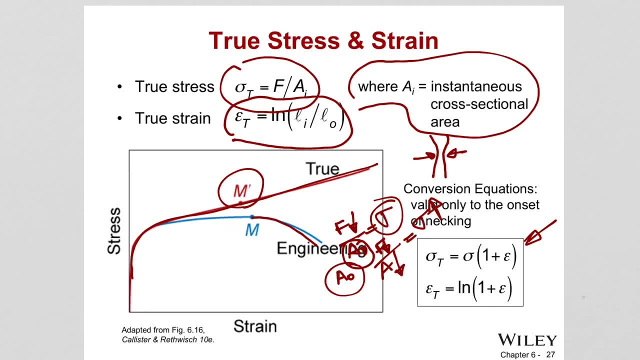 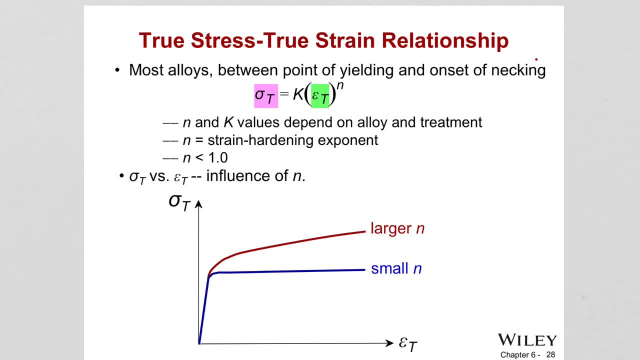 lengths and cross-sectional areas are different in a given time. so, between the point of yielding and onset of necking, alloys are described through this equation. so if we look at the yielding starts here to the necking here, right from this point to that point, this line- okay, this line- is described, the relationship. 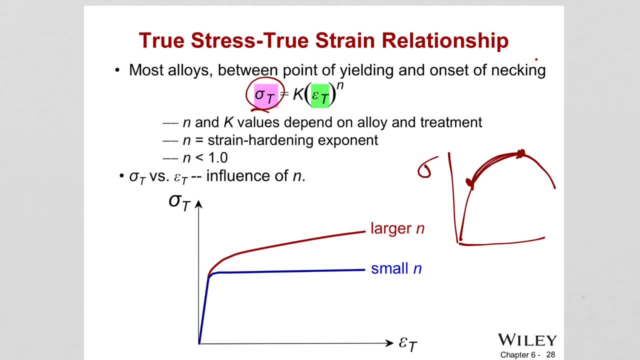 between the stress and the strain. actually this is for the true stress strain curve is described with this equation: how, with stress, the strain is changing and there is a power n, and then there is a constant k, and n and count k are constant. that depends on the material. basically okay, and it is. it is basically what we 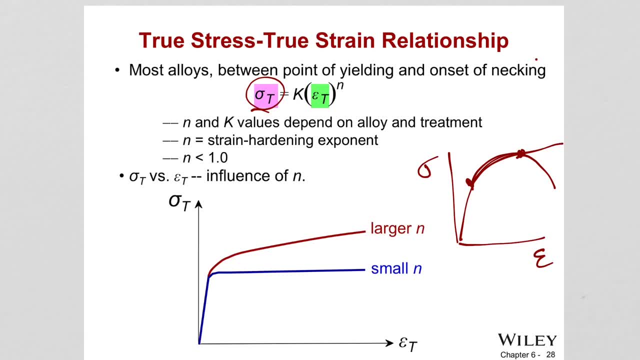 call n is as strain hardening exponent. well, later we're going to see in this region actually what happens as we deform the material plastically. it is getting more, stronger and stronger and we're going to see why that is in the later chapters. and strain hardening basically hardening means. 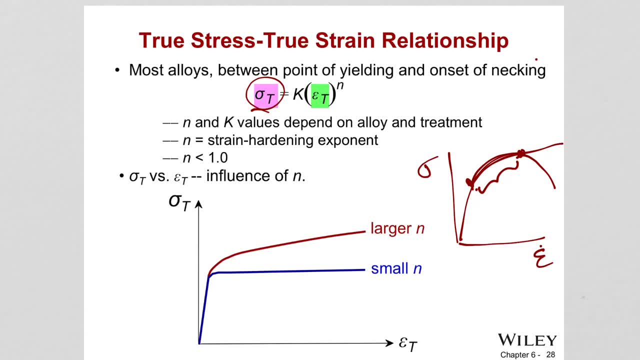 strengthening. with strain the material is getting stronger so that region, the power n, is called strain hardening exponent and it tells us the information that how effective basically the deformation in strengthening that material. So we are seeing through stress strain curve and how materials with small n behaves like and with 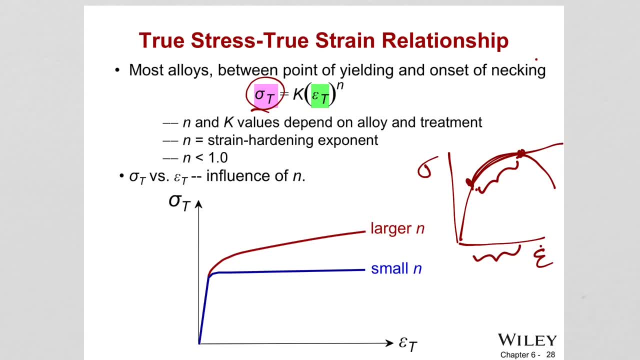 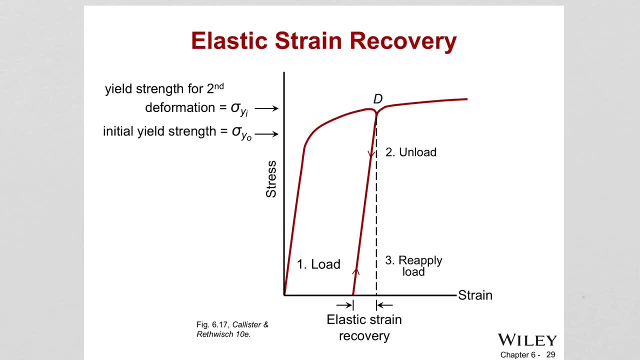 larger n behaves like. So if the n is larger, that means it is. its strengthening is taking place more effectively as we deform the material. So as we taught that elastic strain in the deformed part is recoverable and that graph is defined When we 원- the stress strain curve, we will also show deformed 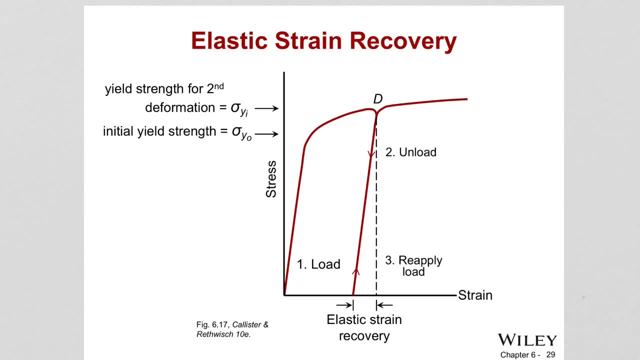 Demonstrating that. So you deform the material up until point D, Collect stress strain data- Okay- and once that happens, you remove the stresses and materials elastic region recovers, go back to original. I mean go back to recovering the elastic strain. What happens? this much plastic deformation remains, but this one, this much elastic is recovered. And I explained to you guys that. 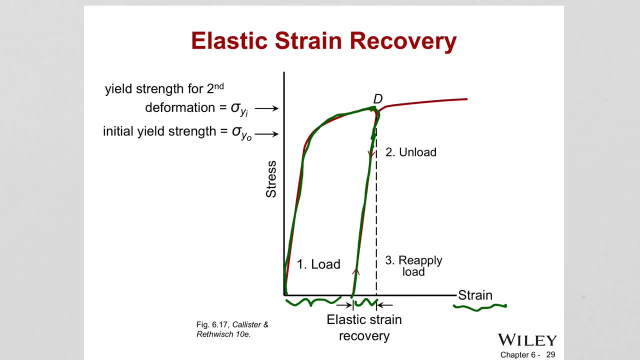 If you actually repeat the same experiment in the same material you apply again. let's choose a color here. If you apply again another, stress again- elastic deformation remains. This time the yield strength will be higher and it keeps deforming plastically. The reason is, once you deform the material right there plastically, the strength of the material increases. 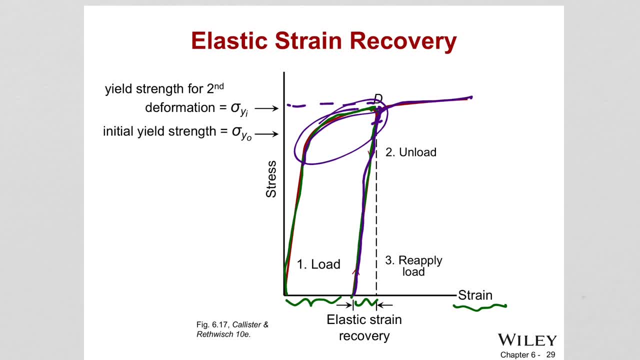 That's why deforming materials actually increases their strength. They call this cold working. At room temperatures. they work on the material like they extrude them or Roll them or do forging like hammering These things. these cold working on the sample actually increases the strength. So once you deform the material, it is getting stronger. 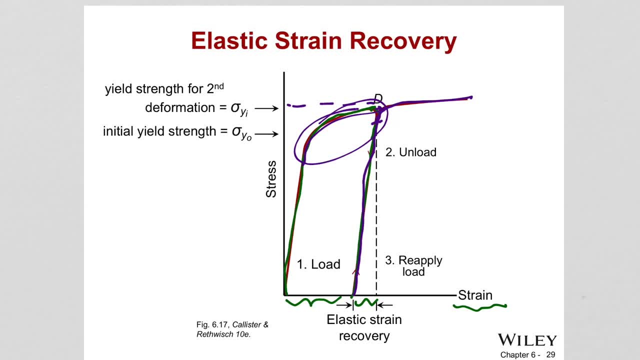 That is the thing you want to keep in mind. So, if you deform a material, it gets stronger. So think about a paper. And you keep deforming them, deforming it, keep deforming it, keep deforming it. at some point it's going to get difficult to deform because, as you keep trying to bend it, bend it, bend it, you are working on the material and you are deforming plastically and the material is getting stronger as you keep trying to bend it, bend it. which have what happens is material actually is getting stronger. 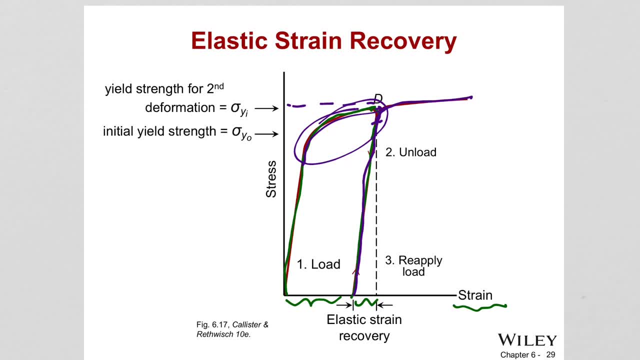 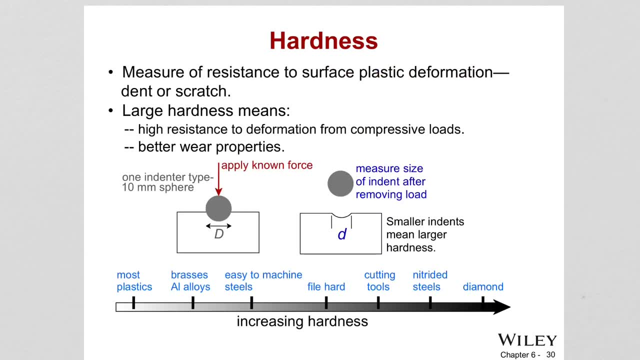 So what is hardest? What happens is material actually is getting difficult to deform because it is getting stronger. So what is hardness? It is again another mechanical property of the materials, So it is the measure of resistance to surface plastic deforming or measure of resistance of the surface tool. 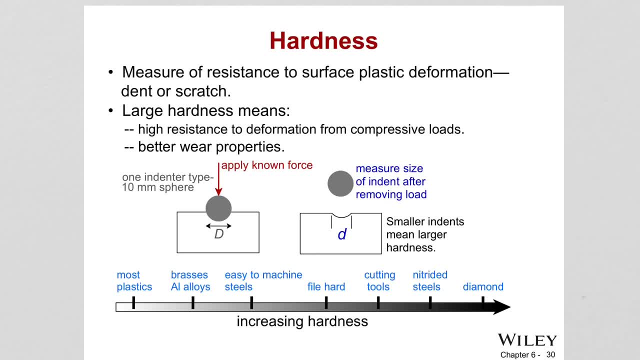 surface opis in general: phase two, then then or scratched. it is something that is very related to the strength of the material. so usually strength and hardness are correlated. okay, so large hardness means it will. the material surface will resist to deformation from compressive loads and it will have better. 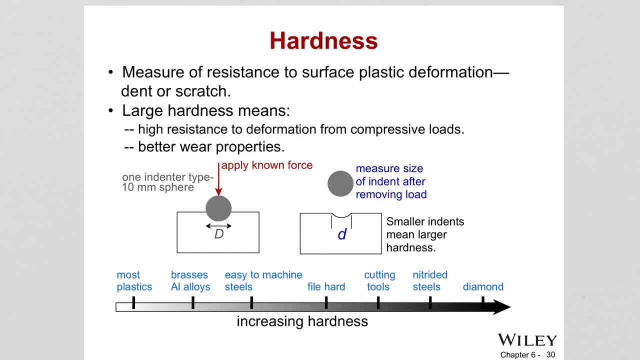 wear properties. so if a material is hard, that means it's better- Have better wear properties. so how it is measured, there are different, different hardness tests and one of them- how the experiment is done, how the Orr hardness is measured, is in the videos I sent you guys. I suggest you to me to watch them to learn how hardness is measured. so there, 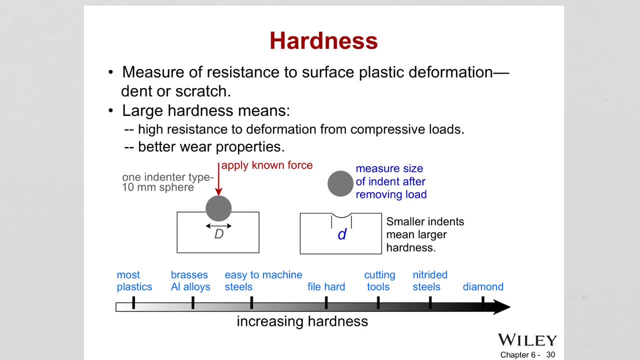 is a particular index, up to six centimeters. we know that it is so different. the different I mean. you know there are different Saskatchewan tests. like the medicine smells and herbs. an indenter, that is, can be made out of steel or other alloys- hard material that is pressed by. 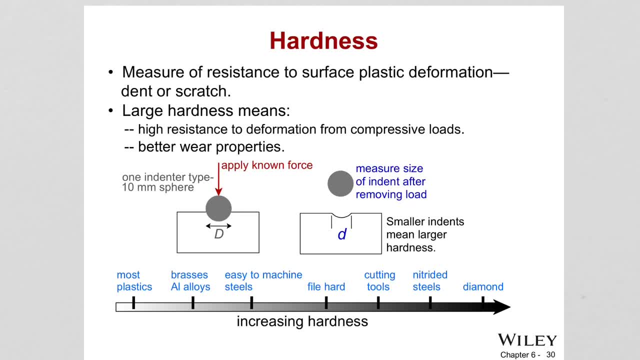 force into the sample. so this is your sample here. okay, you have an indenter which you press on the material and then you measure the diameter of that indentation. okay, after you unload it. so that Diameter will gonna tell you about what is the hardness, will you, of that material. so 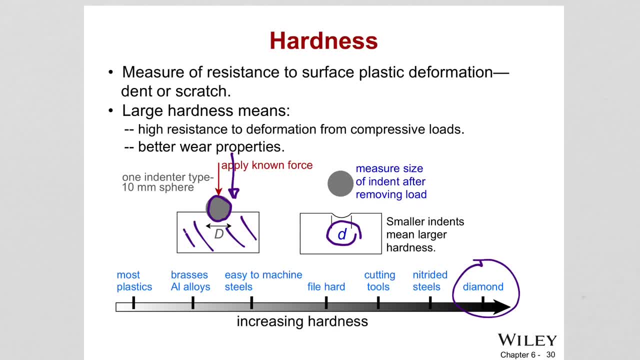 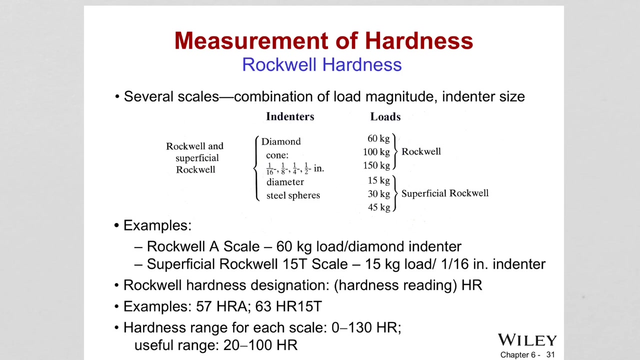 diamond is the hardest ones. and then comes Knight Wright Steel cutting tools and another type of of metal, alloys- metals and alloys, but plastics are in the lowest scale, so they are not hard, but the diamond is the hardest material. okay, so, as i said, there are different types of hardness. 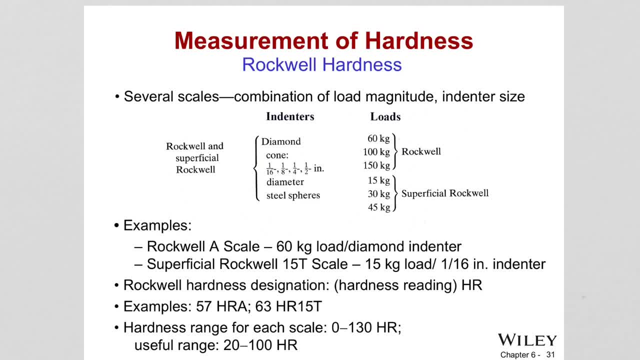 tests depending on what type of indenter they use. so what is the shape of the indenter, what type of loads they apply to? based on that, people came up with hardness tests. one of them is called rockwell hardness, and for rockwell hardness we are seeing we have a diamond indenter or steel and then the 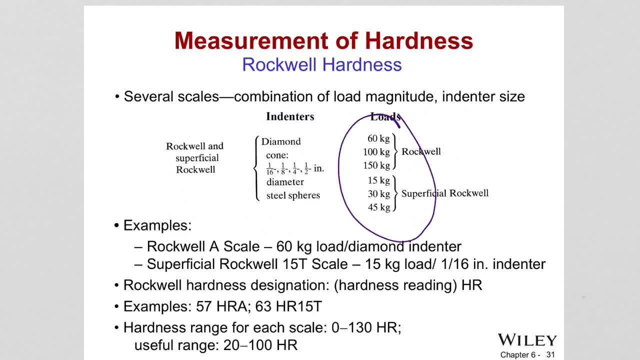 loads that are applied are in this range and based on that, basically, we measure the hardness and we correlate that diameter measured to a hardness volume. in reality, this hardness volume is not exactly a representation of uh, this, what is the hardness? it doesn't have a meaning, the hardness. 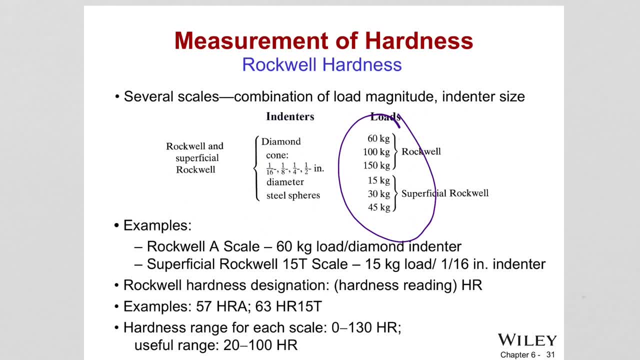 volume is. it is just made up equation to relate between the measured uh indentation parameters to a hardness volume. that's why all the different types of hardness tests are using different equations to obtain a hardness number. so you just call it a number. how they figure out how it's. 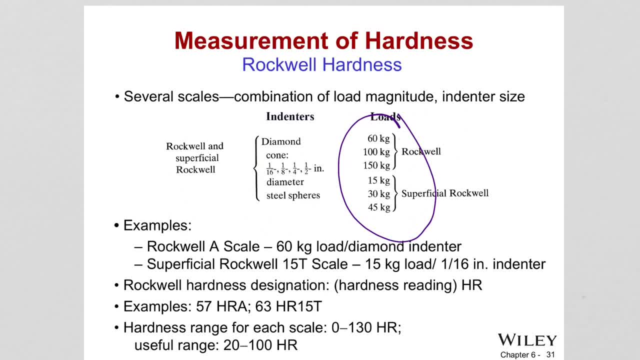 related to the strength is they collect data basically as a function of this hardness number. what is the actual tensile strength, let's say, and then from that data? now, if you collect a diagram, each time you measure the hardness from that diagram, you can go ahead. let's say strength. 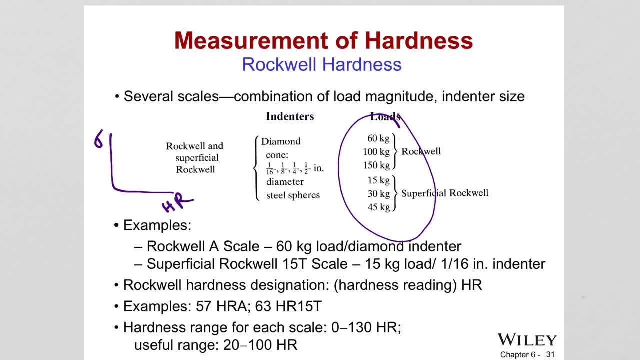 rank hardness number. okay, so each. so you collected the data. let's say the relationship was like that. so each time you measure the hardness you can correlate it to the strength. so, like a calibration curve, you first collect that and then, with the given hardness number, you go ahead and just read the strength. this is how you can relate it. so 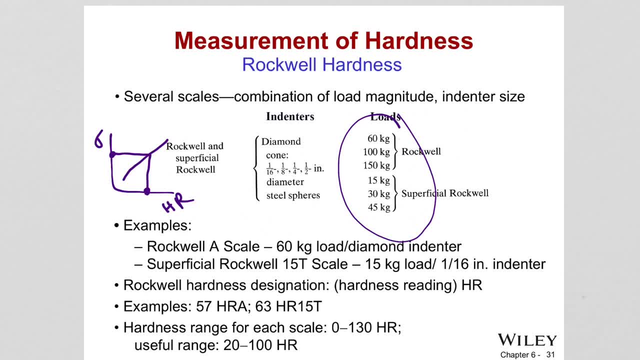 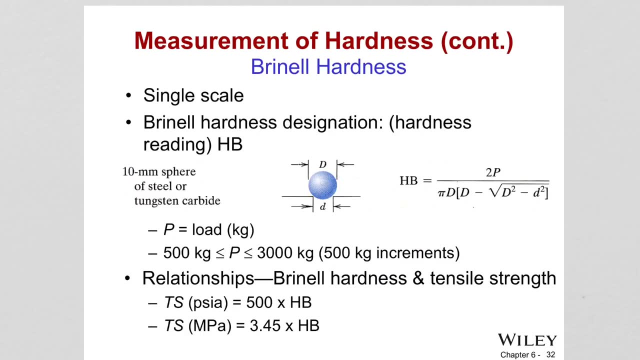 well, this is the branel hardness. next you can order the hardness number. that's how you can attach the problem, if you want to do that. so again, the ran levels are the same, even if they're not the type of test, but just because you actually can connect the- Usually it's multiple test. 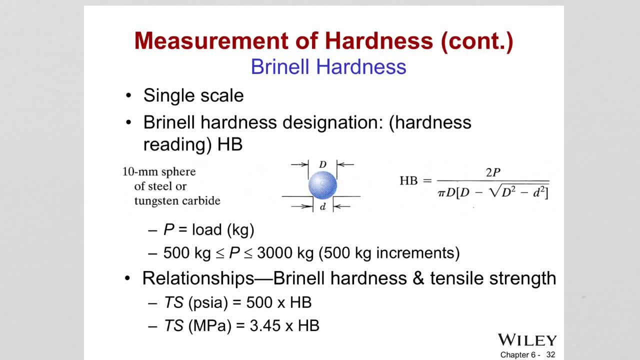 that's why it's called the ryan hardness number. so this is ryan hardness number here. but the hardness number, how it is measured, hp, is the brine hardness. this one uses a sphere of tungsten or tungsten carbide and or a steel indenter to push on the material and the d capital d is. 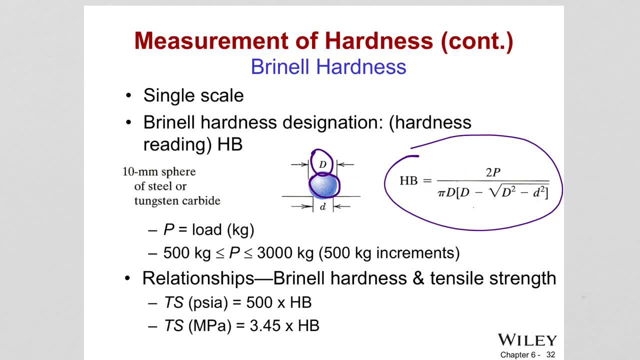 basically the diameter of that sphere. it is 10 millimeter and d is the indentation diameter. that's why, if you plug in these numbers in these equations again, this equation is different for each different types of tests. for brine hardness, you use that equation to calculate the hardness. 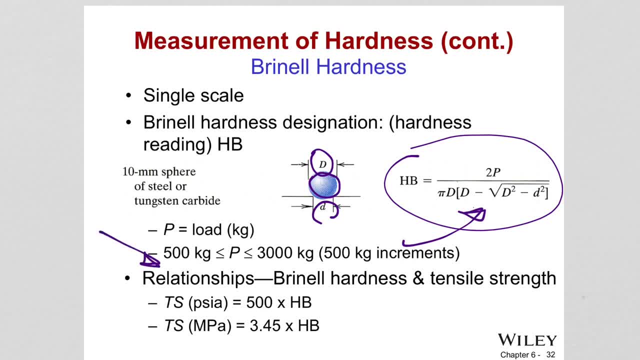 number and we are given the range of loads that are applied. and there also has been found a relationship between the tensile strength and calculated brine hardness values and these equations are given here, depending on which units you want to use, if you're gonna use psi. 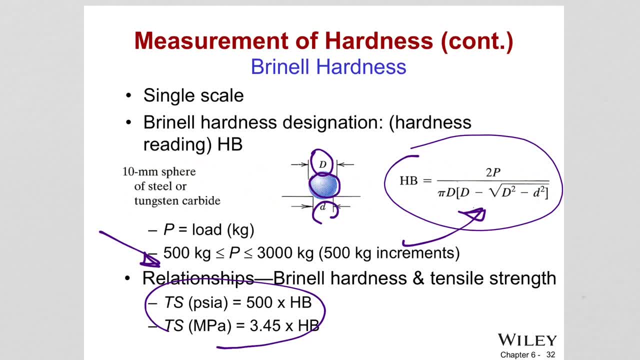 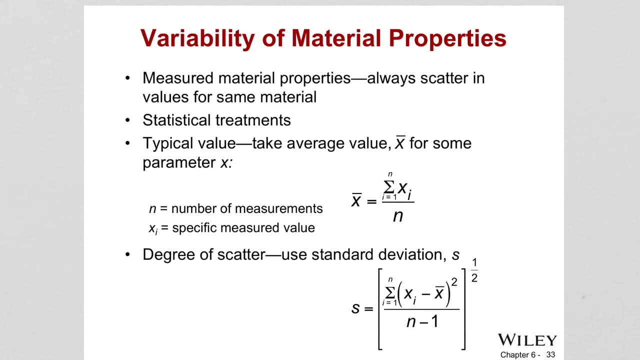 psi a or np m, mega, megapascal, depending on that. you just have to multiply the brinal hardness to certain number and you calculate the tensile strength. okay, so this relationship is important, all right. so the problem arises when we do testing, because even we are sampling the same material. each test will not. 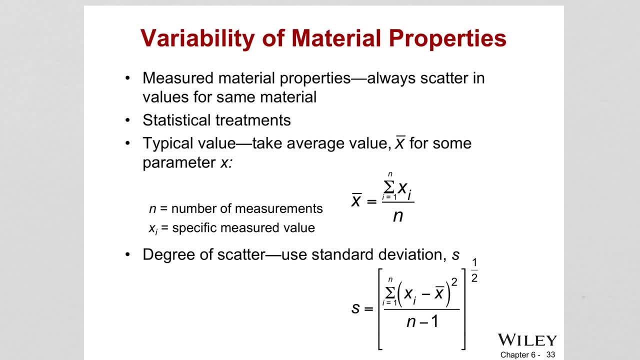 going to give us the same result. okay, there will be small variations it between the results of the test, even for the same material. therefore, we need to approach the problems with some statistical treatments. how do we take the average volume, let's say, how do you measure the yield strength? 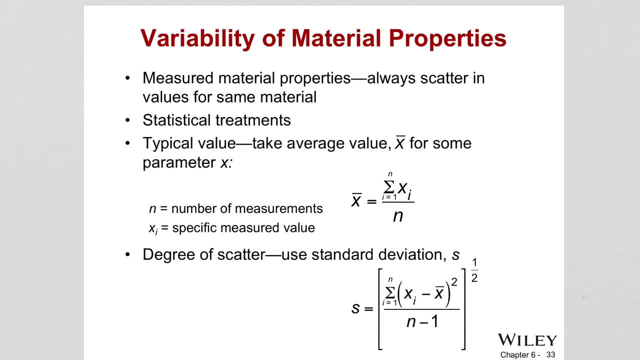 if the test gave you multiple yield strength for the same material, how are you gonna get that yield strength? you need to average it right and, being the number of measurements, X, B, X, I, being the specific measured volume, just average them. and also standard deviations, how the data is scattered, how. 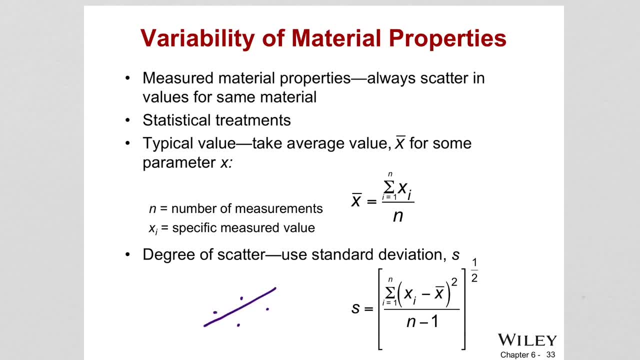 much it's scattered. let's say, this is the average and the data is scattered everywhere, right so, how it? how much it is scattered? there's basically this is doing. basically, you basically need to square it, because how, what is? what are the distances to the mean volume? right so, basically, average volume, this is the average. 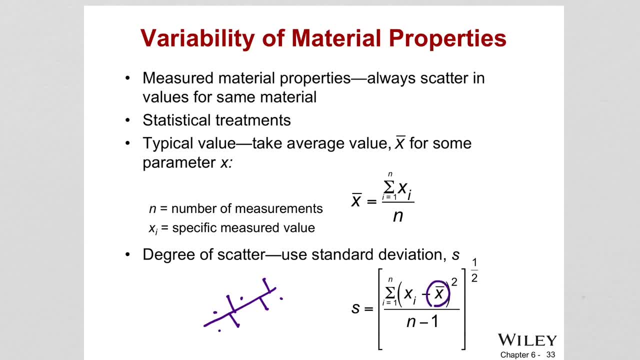 volume. remember so each data, how it is changing relative to the average volume and how it is changing relative to the average volume. that can be a negative change or positive change. therefore we need to square it to get rid of that negativity and then do square root of the overall and then 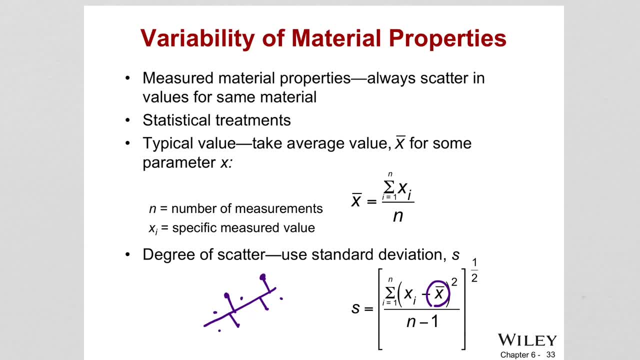 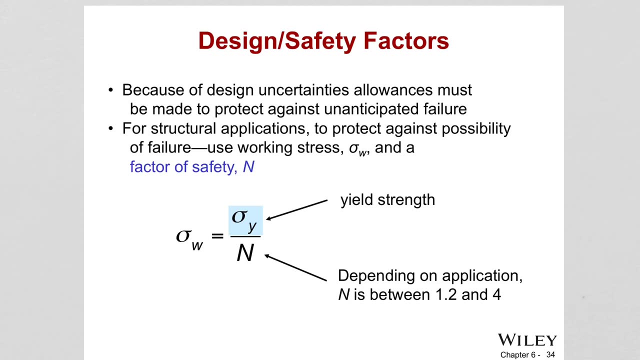 divide it to basically how: n-1. okay, you start from 1 and then do the experiment n times, right? so that's it basically. so there are some safety factors because there can be uncertainties and we need to protect to make sure there is not gonna be a failure. at least make sure of it, I mean, at least try our best, right. so for structural 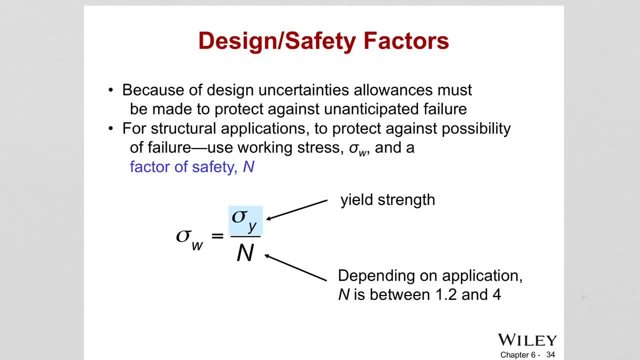 applications to protect against the failure, use working stress, Sigma W and the safety factor. so the safety factor relates the work working stress to the yield strength of the material and the yield strength of course needs to be uh bigger than the working stress, um, because this will ensure that the failure, the possibility of failure, will decrease. 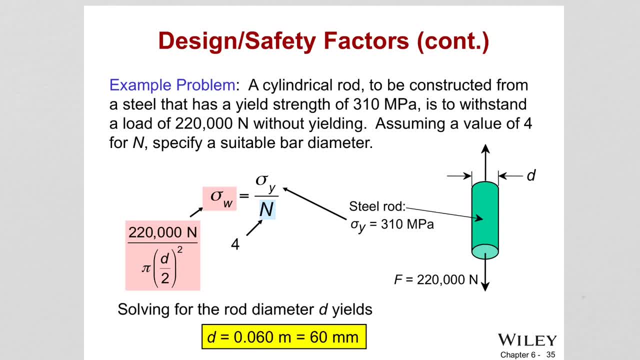 so here is an example: we have a cylindrical rod and constructed from steel and the steel's yield strength is 310 megapascal is to withstand. it will withstand a load of force of 220, 000 Newton without yielding. okay, assume a volume of 4 for the safety factor n and specify a suitable bar diameter. okay. so this 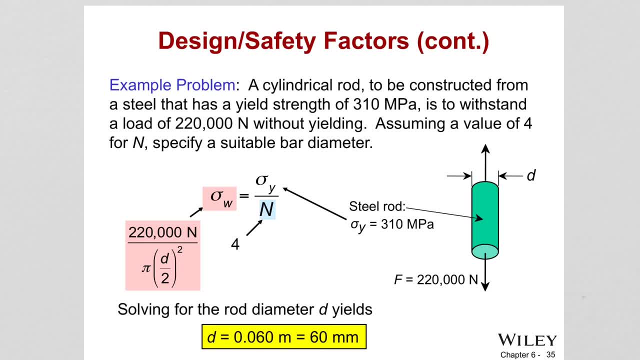 a material is going to be exposed to uh loads, the force of 220 000 with a certain area right. that is the working load, working stress and the yield strength of the material is 310.. so this is given to us, we plug into the data the equation, and n is assumed to be four. uh, the pressure goes down until C4. we put the pressure left by Moon, which will be 2, and anar is assumed to be A 4. so this is given to us, we plug into the data the equation, and n is assumed to be four. prank Ihr, and that means Ctrl, and N are assumed to be all right, so that means recordings. then we need to measure this. that's absolutely observable, even when you measure it. so maybe there is a area which is 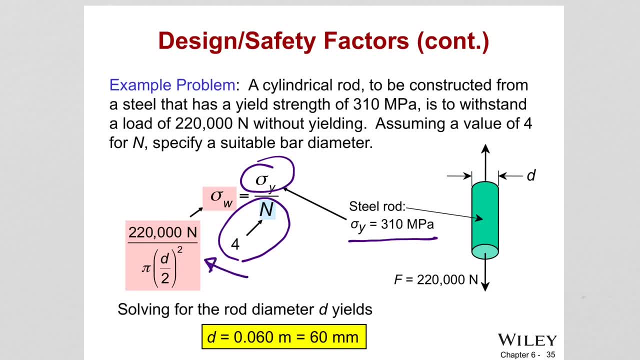 So from that you can calculate, because working stress is the force over area, basically, and area is diameter over 2, is the radius, radius squared right, pi r squared, pi v over 2 squared. so this is the area and this is the force, and from this equation you can calculate the 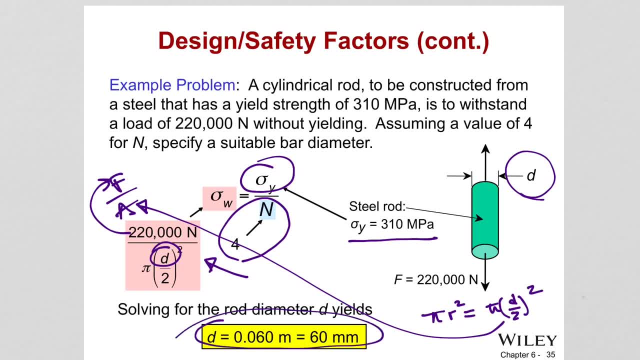 diameter. that is that this steel bar needs to be constructed from. okay, So basically, you are ensuring that the working yield strength of the material is 4 times of that working stresses. This will it will not. you will try to lower the possibility of failure with this safety. 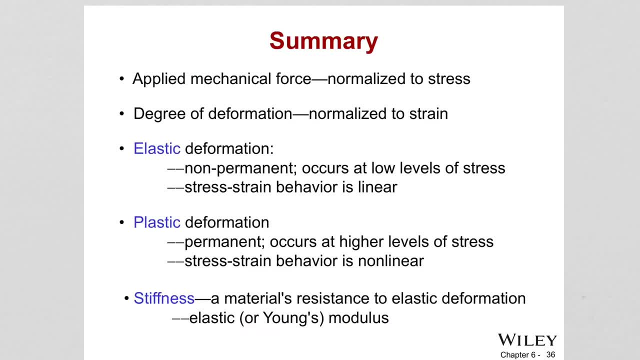 factor. That's it, Okay. So, in summary, we looked at how the materials are reacting to mechanical forces and how much they deforming. we said it is. it's giving us stress and strain data. and elastic deformation is non-permanent, occurs at low stresses. it's linear. 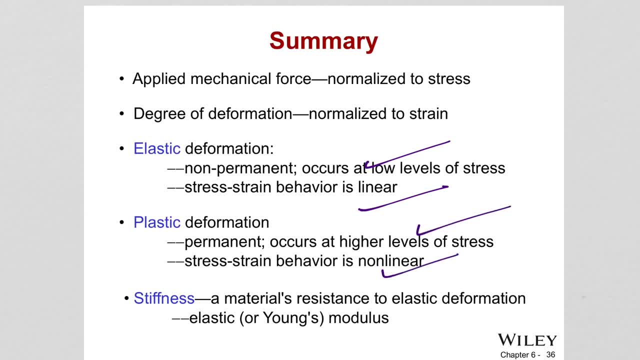 Plastic deformation occurs at higher stresses. it's non-linear Stiffness is a property of material Due to the atomic bonding strength. it is determining the resistance to elastic deformation. If the material is difficult to deform elastically, we call it stiff and and try to deform a. 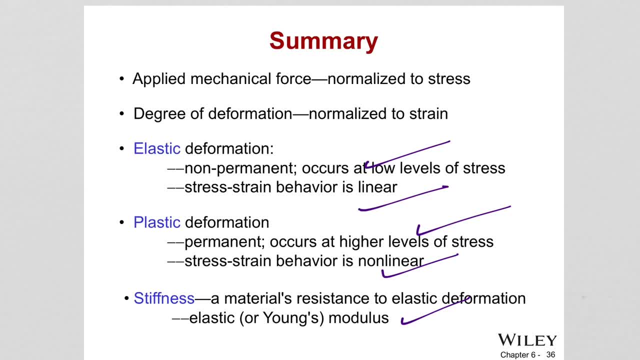 steel bar, for example. with your bare hands right it's difficult, But try to deform a material with low modulus like a rubber. you can easily deform it elastically. So strength was two types: Yield and strength, Tensile strength. 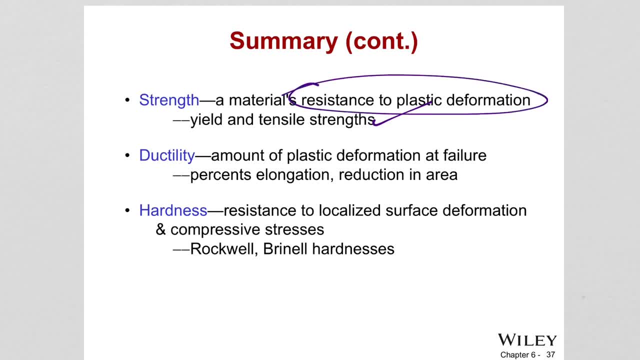 It was the material's resistance to plastic deformation. Ductility is how much we can deform the material to what extent until it fails. We calculated from percent elongation or a reduction in the area. Hardness is resistance to scratches, the surface, deformations and under compressive stress.